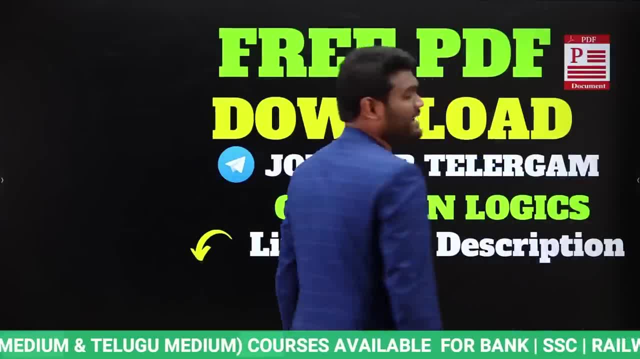 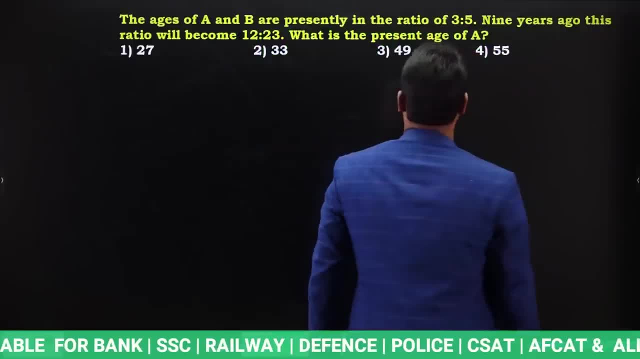 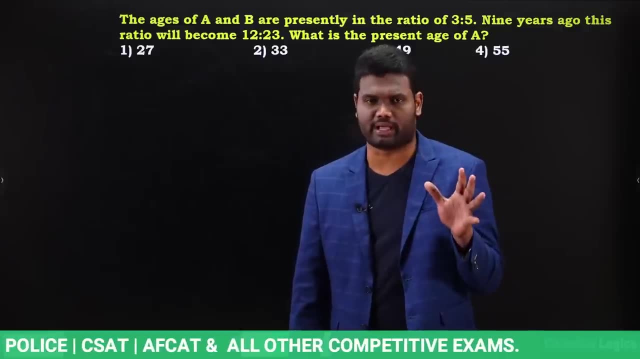 link in the description And if you want to download free PDF materials, you can join our Telegram group. We have provided our Telegram group link in the description, So in this video we are going to discuss questions from topic ages. Actually, ages is one of the simplest topic. 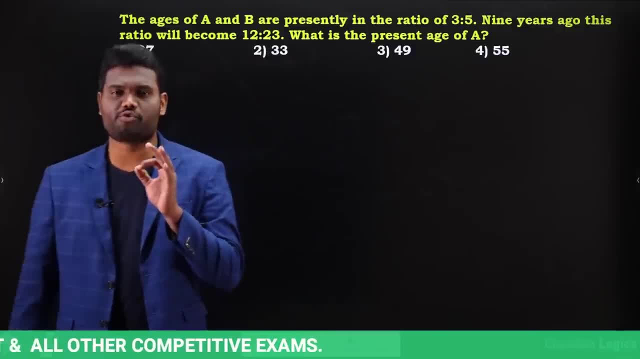 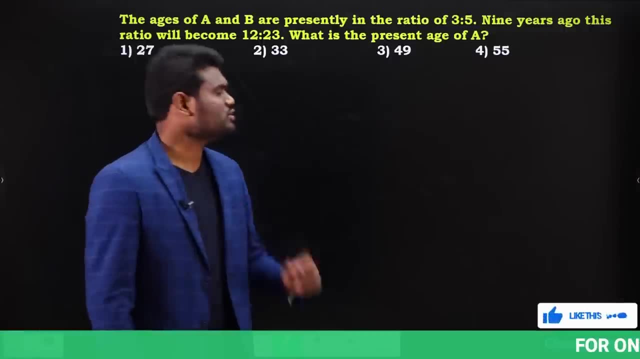 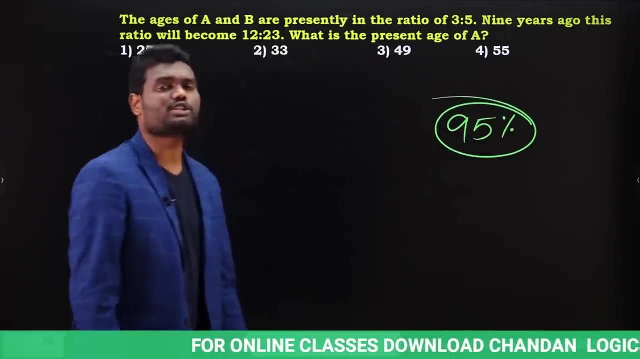 And, truly speaking, 95% of questions from topic ages can be answered without using your pen and paper. Yes, without using your pen and paper, 95% of questions can be solved very, very easily, in just fraction of seconds. I am going to share the wonderful technique. 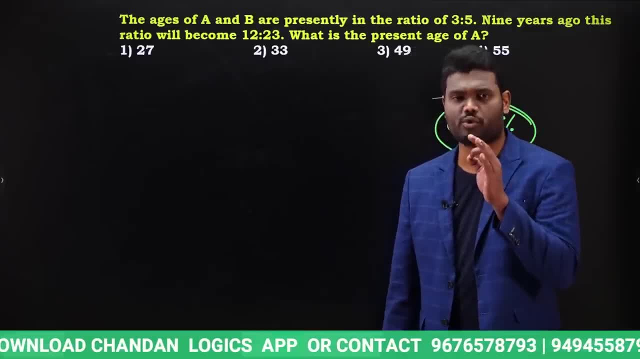 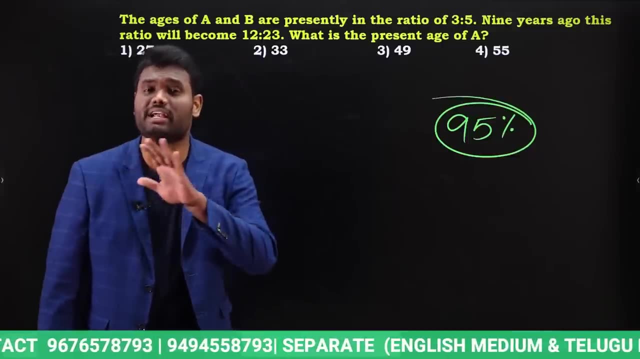 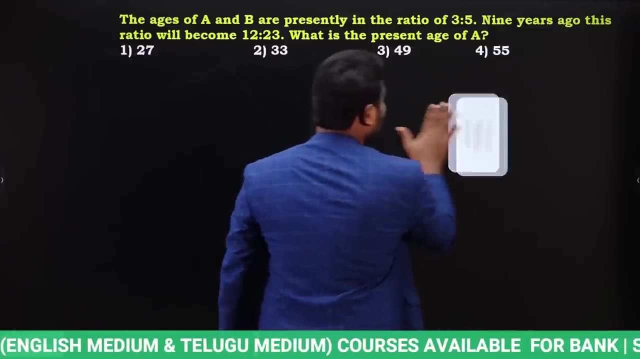 where you can solve 95% of questions from topic ages without using your pen and paper. So just watch the video completely and you're going to get complete idea how to solve questions from ages without using your pen and paper. Okay, And this is very important topic And from this topic you're going to get questions frequently. 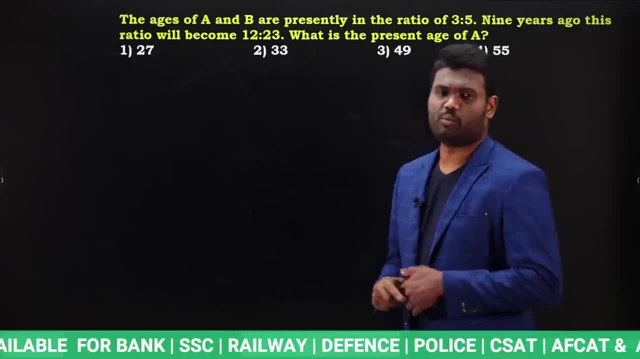 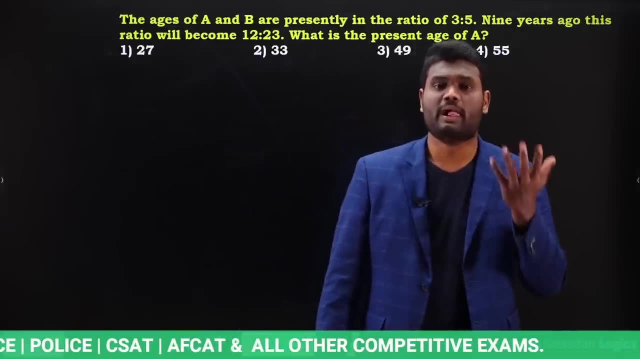 in every COMT2 exam. whatever the examination you're going to get, whether it is bank exam or SSC exam, or railway or defense or CAT or AFGAT examination, whatever the examination may be, definitely you're going to get questions from topic ages. Okay, Look here. Here we have a. 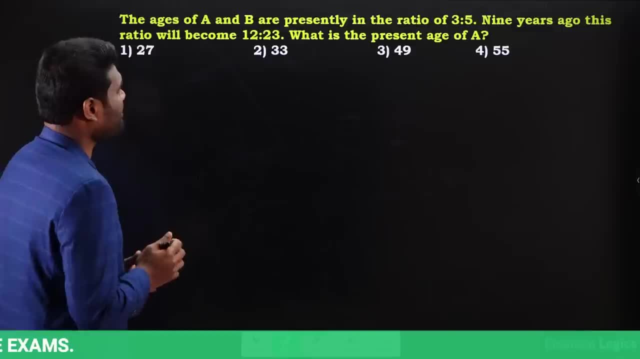 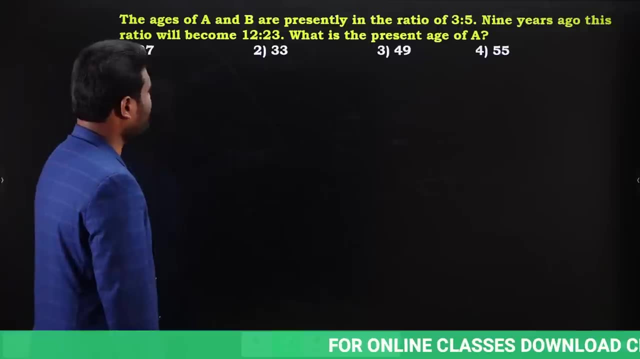 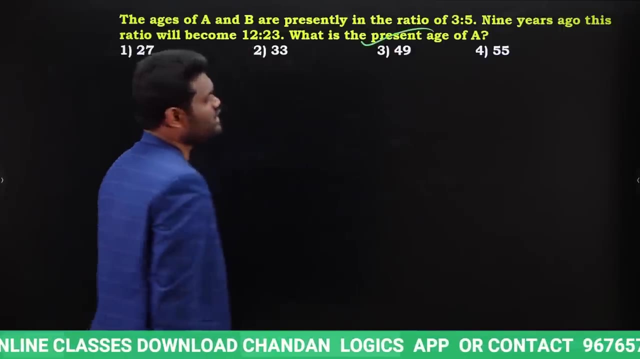 question. The ages of A and B are presently in the ratio 3, ratio 5.. Nine years ago this ratio will become 12 ratio 23.. What is the present age of A? So we are supposed to say what is the present age of A? And don't forget, in this video I'm not going to discuss complete concept. 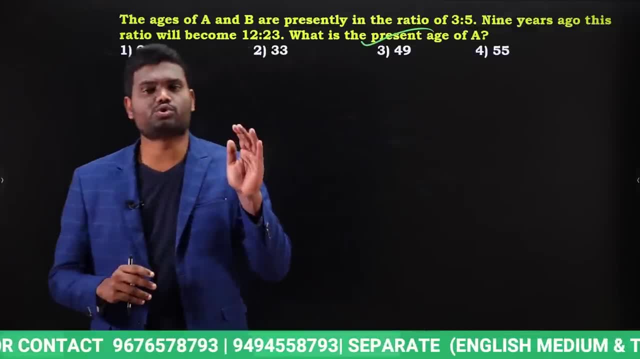 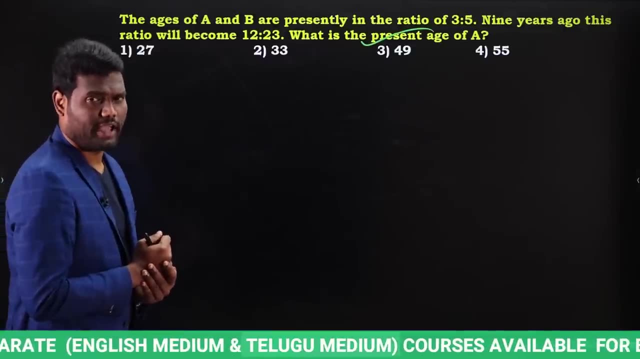 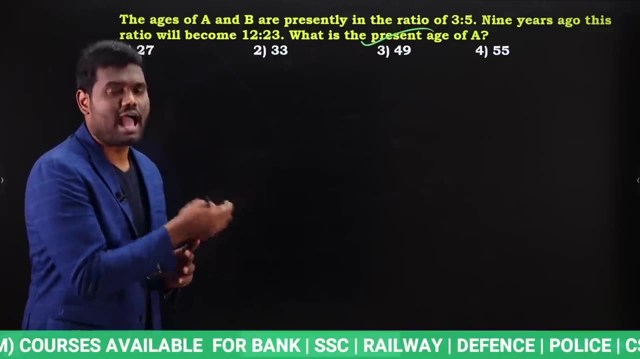 I am going to share you smart approaches to solve questions in examination point of view. Okay, Now look here We are supposed to say present age of A. Actually, this question can be solved in several ways. First, what generally Most of the students do. I am going to show that. Observe carefully What most of the students will. 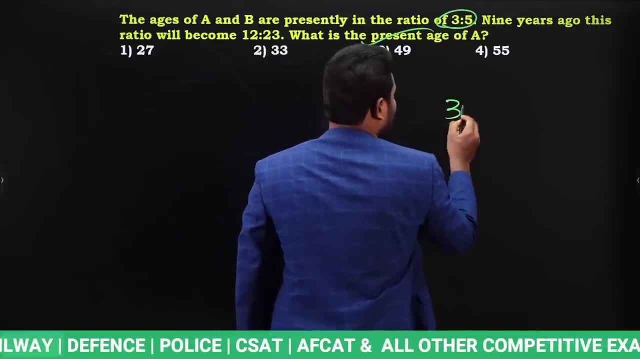 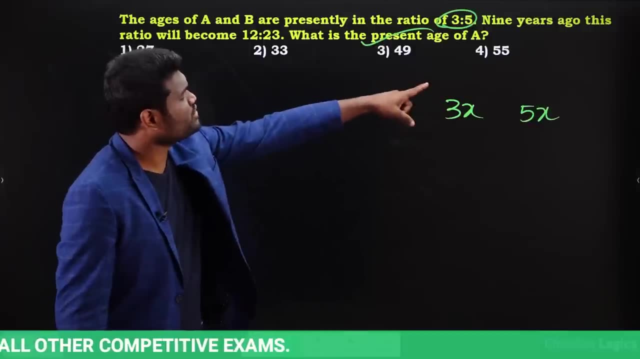 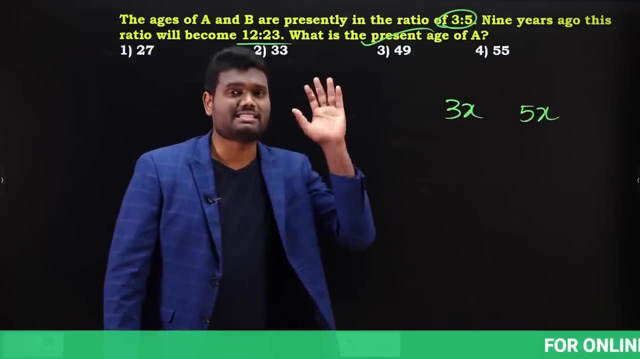 do is they will take present ages as 3x 5x. Yes or no Present ages 3x 5x? Next question said nine years ago. this ratio will become 12 ratio, 23.. Nine years ago means I have to subtract. Yes. 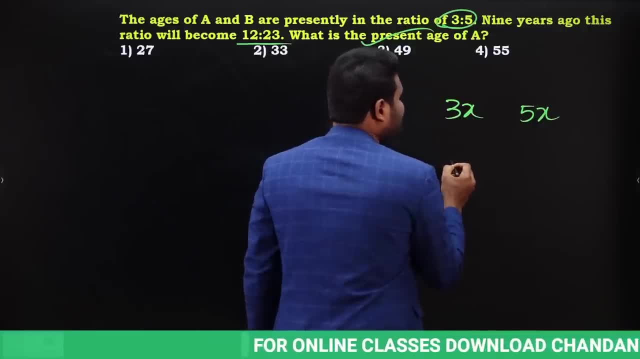 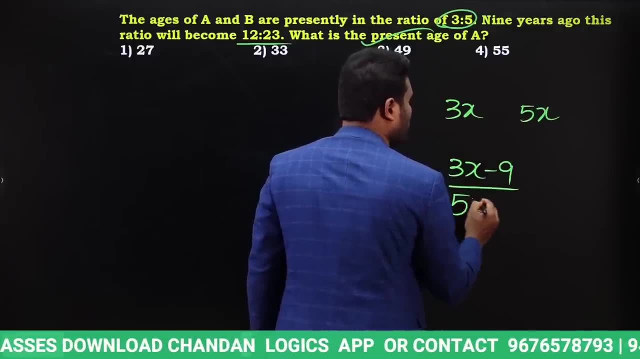 or no. Nine years ago means I have to subtract. If present age is 3x nine years ago means it's should be 3x minus nine. If present age is 5x means nine years ago, means it should be 5x minus. 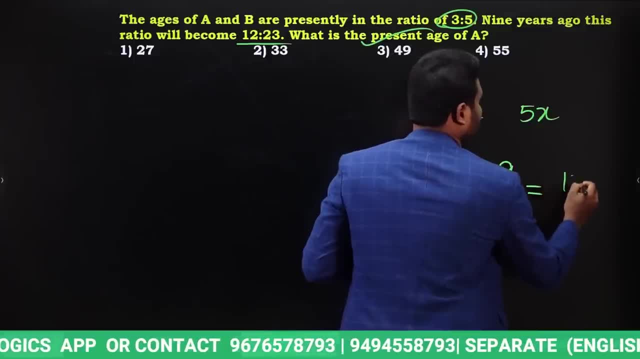 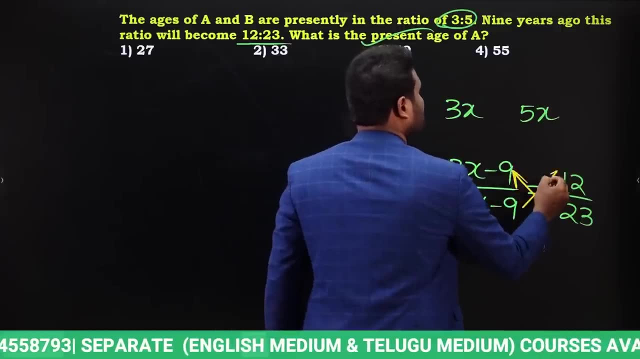 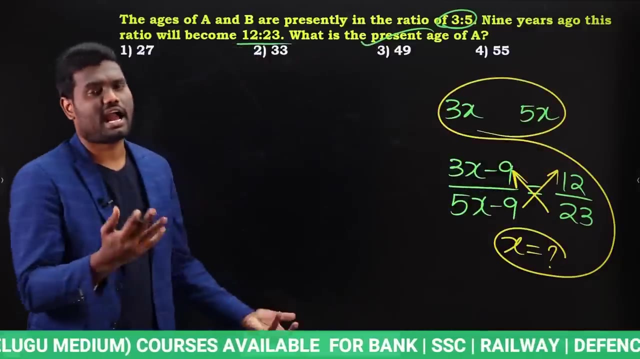 nine, Nine years ago. what is the ratio? Ratio is 12, ratio 23.. Yes, Now what we have to do? We have to do cross multiplication. Once we do cross multiplication, we will come to the value of x. Once we know the value of x, then we can say A's age and B's age also. Yes, Now, this is how most 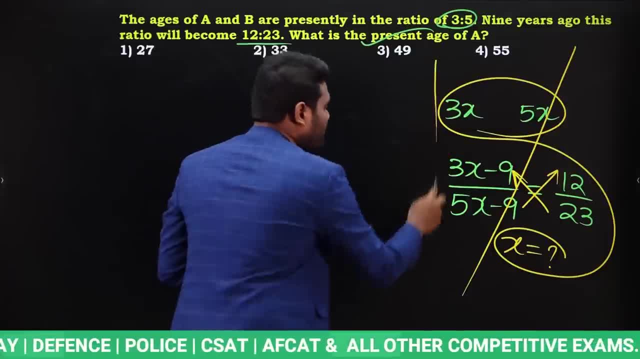 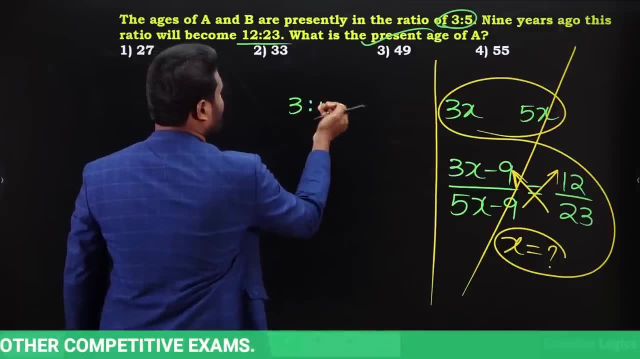 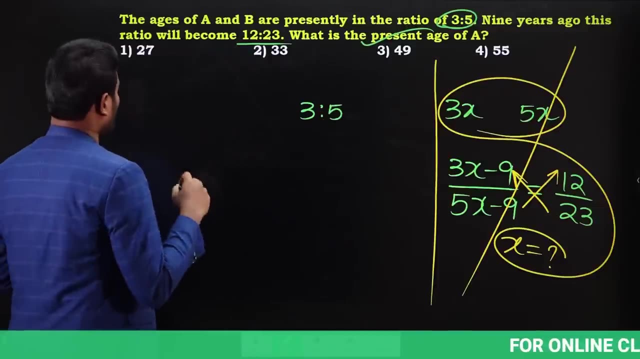 one way to solve the question. Okay, One more way. One more way to solve the question is: observe carefully: Present age ratio. is what Present age ratio is 3 ratio, 5.. Yes or no? Present ages ratio is 3 ratio 5.. Nine years ago this ratio will become 12 ratio 23.. Nine years ago, ratio is 12. 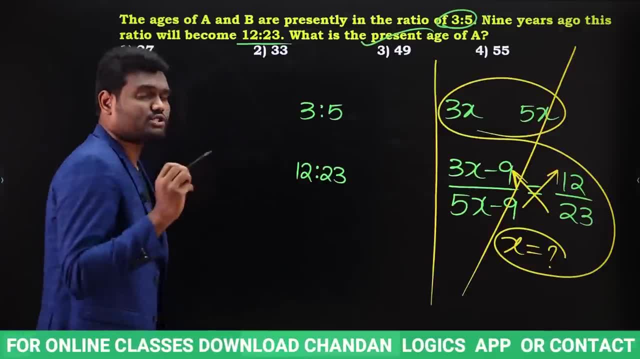 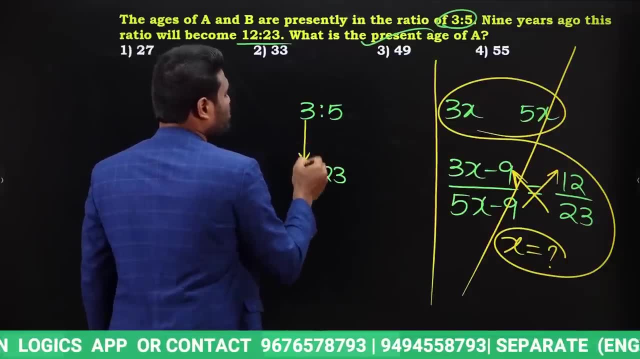 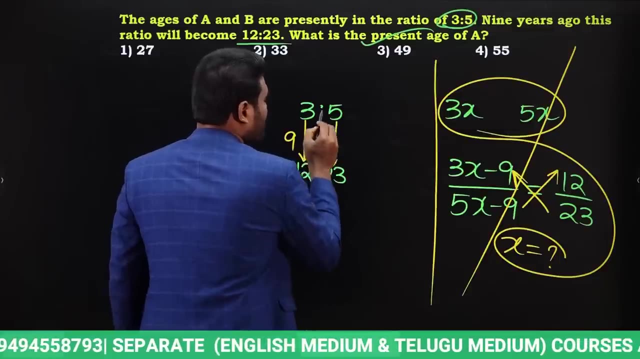 ratio 23.. Now observe here Most of the students they will try to do with parts. When they are trying to do with parts, look here: What is the difference here? 3x12 difference is nothing but nine, Okay. Next, similarly, if you observe here 5x23, what is the difference? 5x23 difference is: 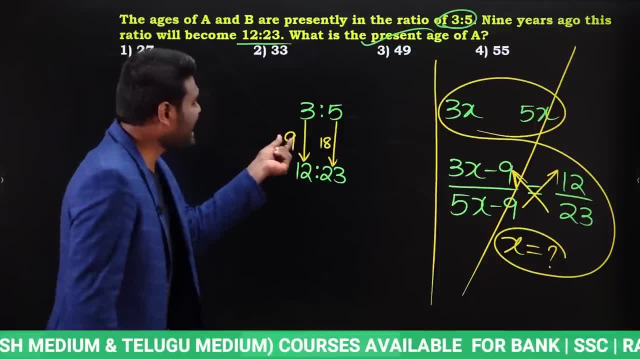 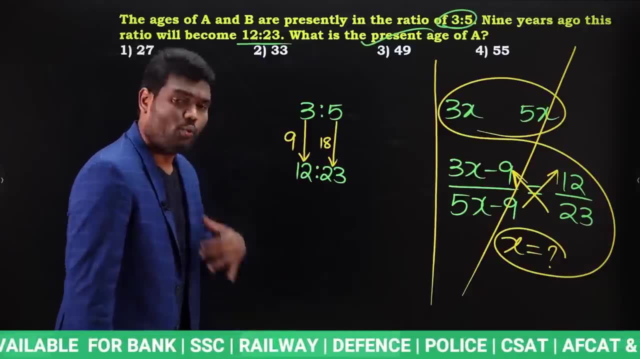 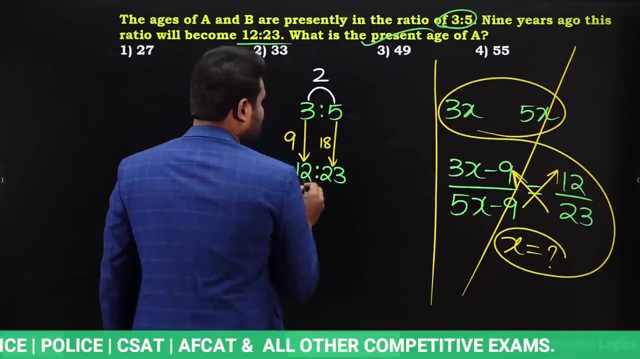 nothing but 18.. Okay, Now observe here: This is nine parts, This is 18 parts, which means parts are not same. When parts are not the same, we have to make them same. How to make them same? Just take above difference: 3x5 difference is what Two? Next, 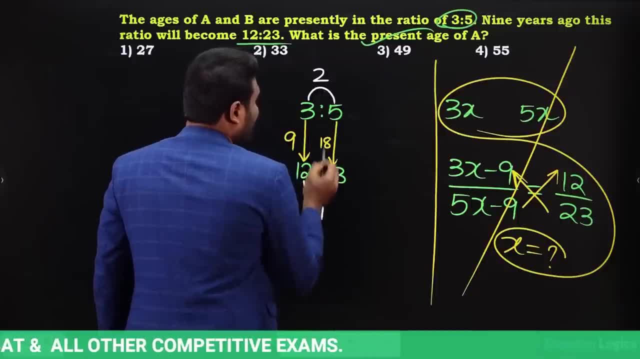 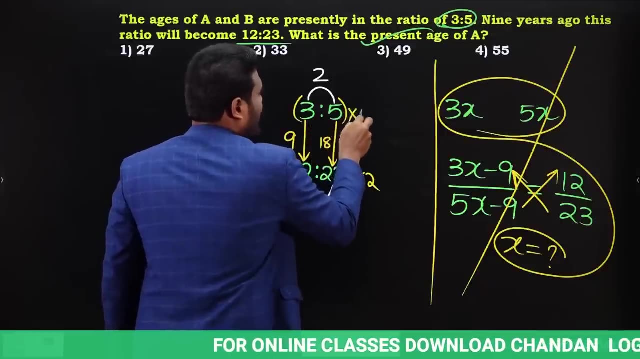 take below difference: 12x23 difference is what? 11.. Take above difference, take below difference And next what you have to do is multiply above difference below. Multiply above difference below, Okay. Next, similarly, multiply below difference above. Now once, if you are going to do this, 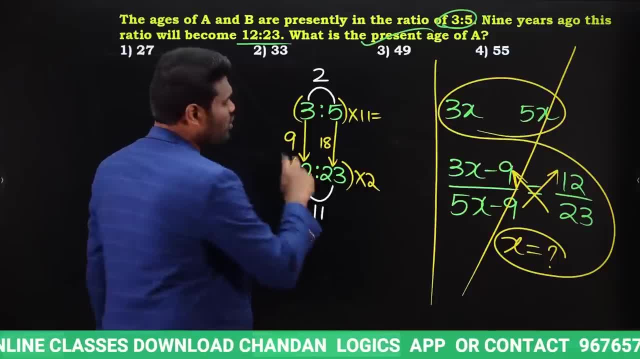 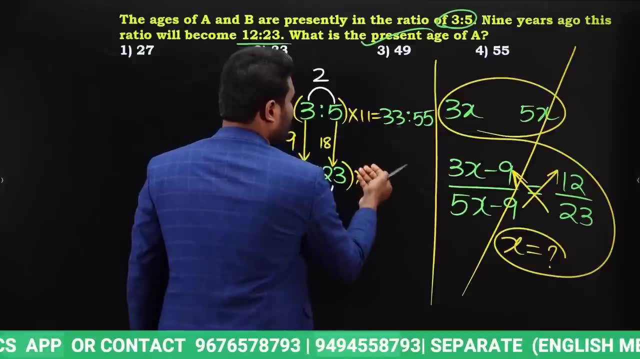 then automatically, parts is going to become same. If you want, you can check: 3x11.. Now, this is going to be 33.. 5x11.. Now, this is going to be 55. Okay. Similarly. 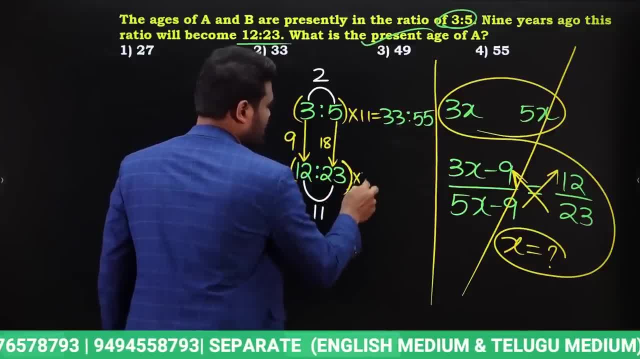 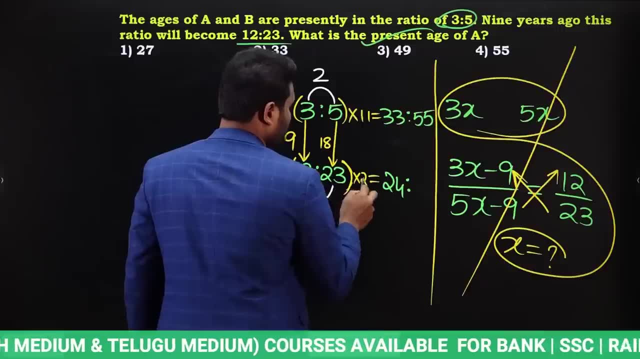 observe here. Similarly, if you observe here just a minute, this is 3x2.. So if you observe here, 2x12.. Now this is going to be 24.. 23x2.. Now, this is going to be 46.. Okay, Now observe here. 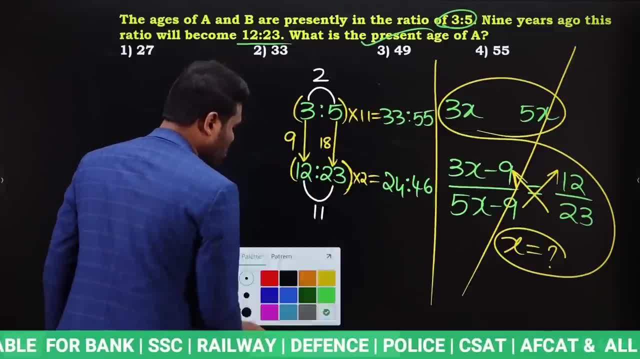 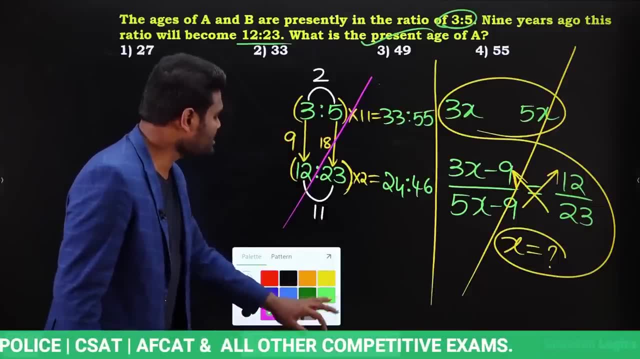 carefully. Once after getting the new ratios, you have to neglect old ratios. Once after getting new ratios, you can neglect old ratios. Now check whether the parts are same or not. Now observe here: 33x24 means difference is going to be 24.. Now check whether the parts are same or not. 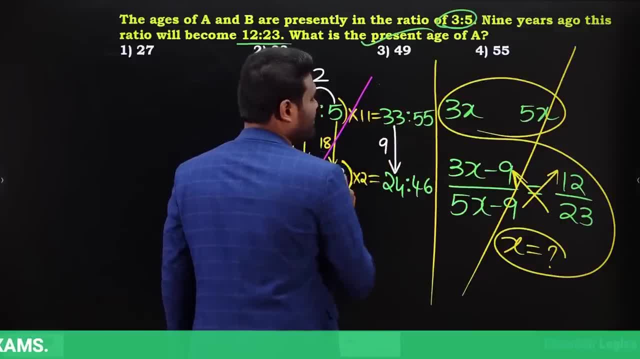 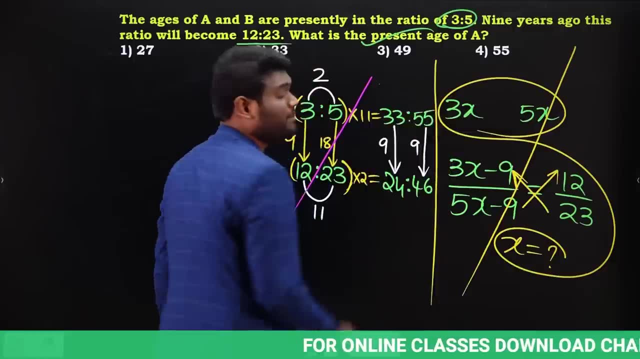 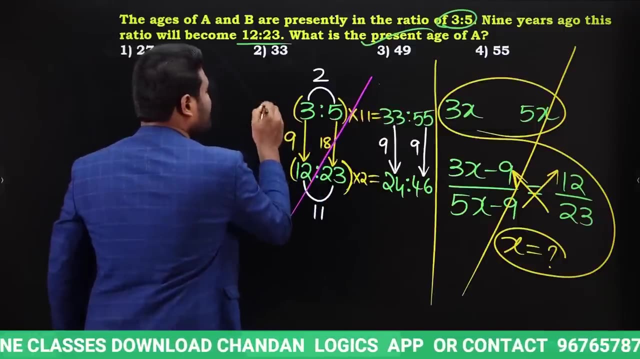 be how many parts? 33, 24 means difference is going to be 9 parts. yes, similarly, 46, 55, 46, 55 means difference is going to be how many parts? 9 parts, yes. now observe here: parts are same. yes, parts are same and this is nothing but present ratio. yes, this is present ratio. this one is what this is. 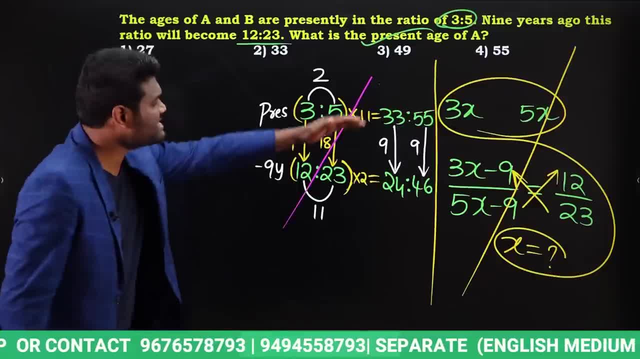 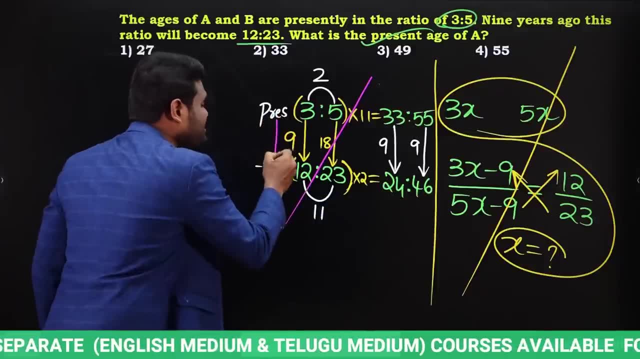 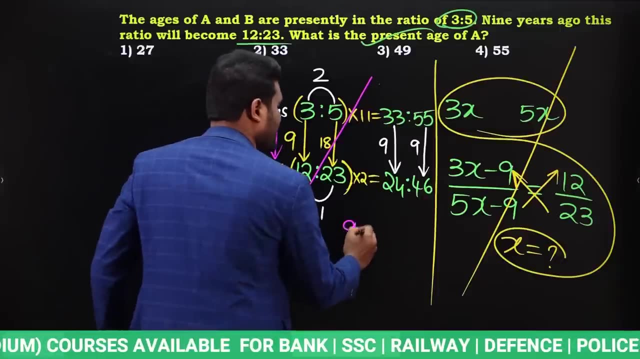 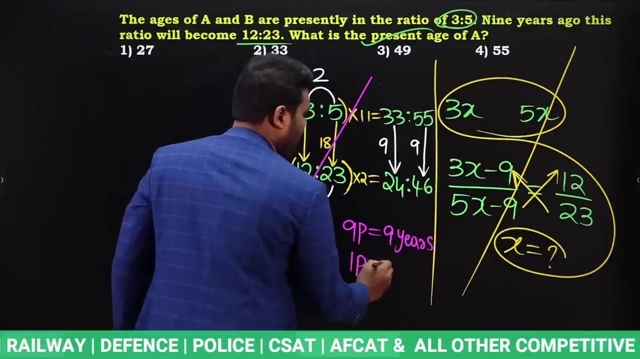 9 years ago ratio, which means difference in parts is 9 parts. yes, difference in parts is 9 parts. difference in ears is 9 ears, yes, parts difference is 9 parts. ears difference is 9 years. so i can simply say 9 parts is equal to 9 years. yes, if 9 parts is 9 years, we can say 1 part is equal to. 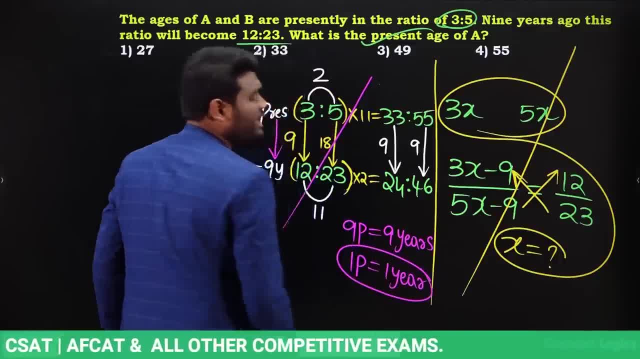 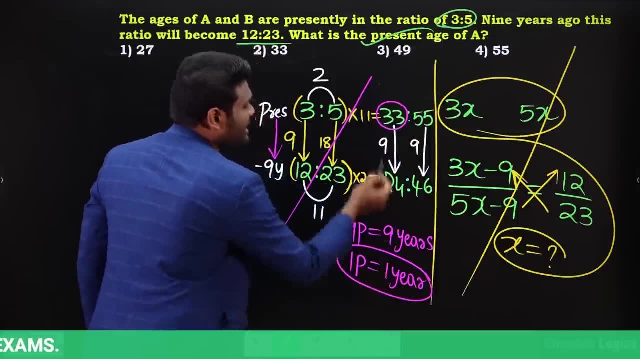 1 year. if 1 part is 1 year, we need to know present age of A. Present age of A is nothing but 33 parts. So if one part is one year, 33 parts is going to be 33 years. So we can say answer for this question is going to be 33 years. 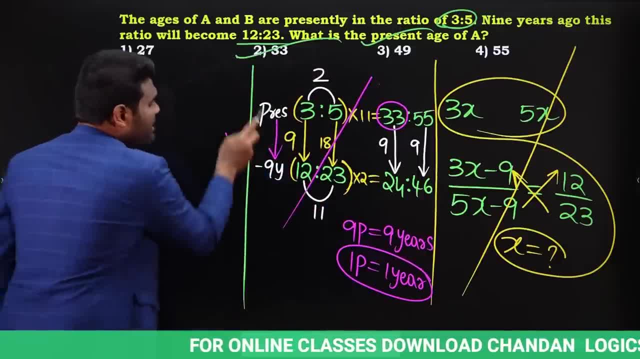 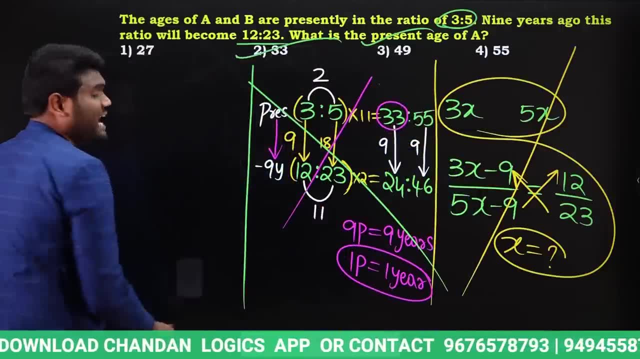 Yes, Now, this is one way to solve the question. Even if you solve in this way, it is going to consume time in examination. Yes, We have one more way. Observe carefully One more way, And after this I am going to say how to solve the question. just by looking at the question Just. 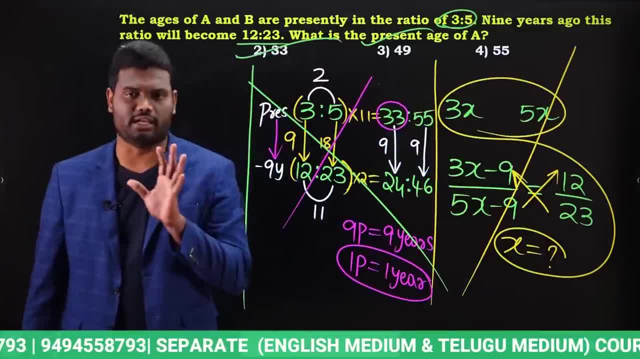 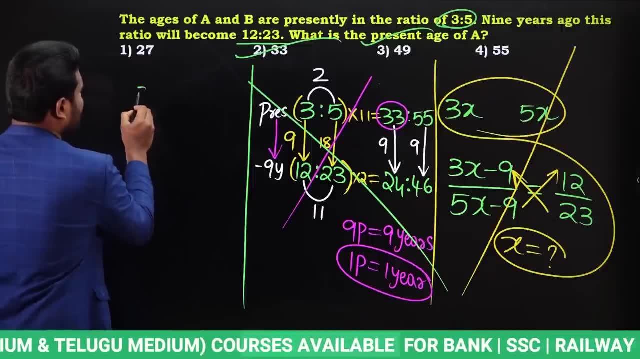 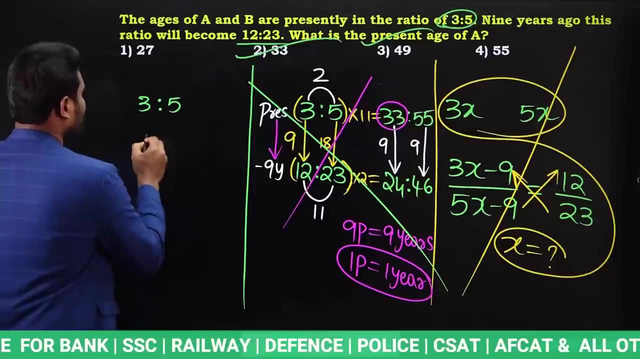 by looking at the question how to solve age-risk questions very easily. Okay, Observe carefully One more method. One more method to solve this question is present. age-risk ratio is what Present age ratio is 3 ratio 5.. Present age ratio: 3 ratio 5.. 9 years ago ratio will become 12 ratio. 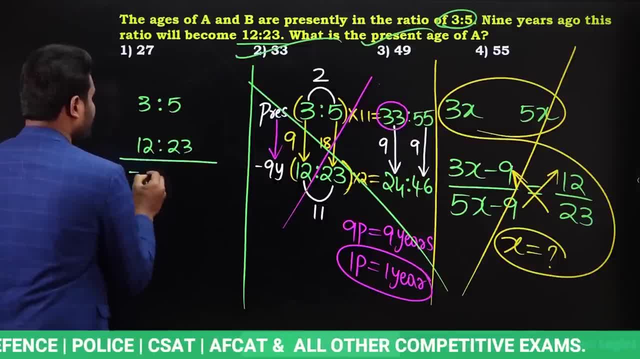 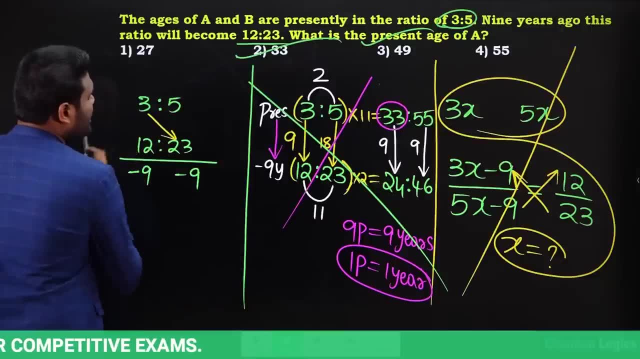 23.. Yes, So 12 ratio 23, when 9 years ago, As it is 9 years ago, minus 9,, minus 9.. Okay, Now what you can do is do cross multiplication 3 into 23.. 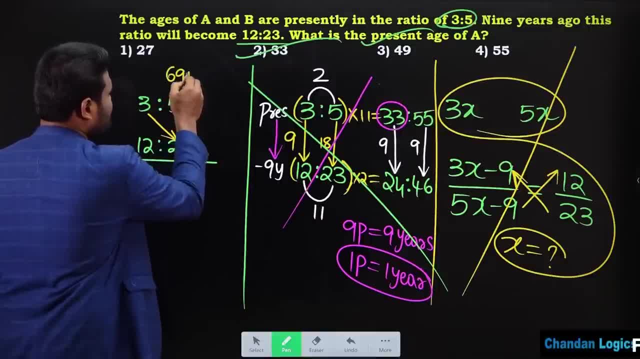 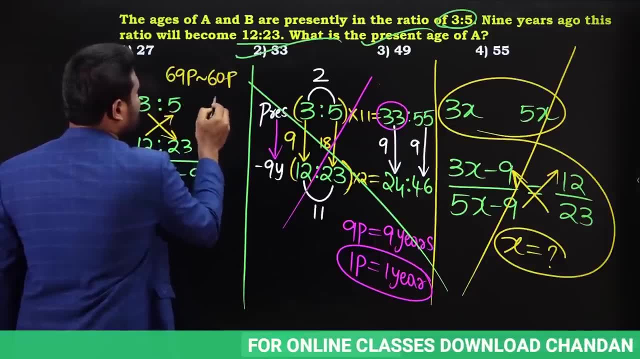 What is 3 into 23?? It is going to be 69. So 69 parts. 12 into 5. It is going to be 60. So this is going to be 60 parts. Now, 69 parts. 60 parts means difference is going to be how much. 9 parts. 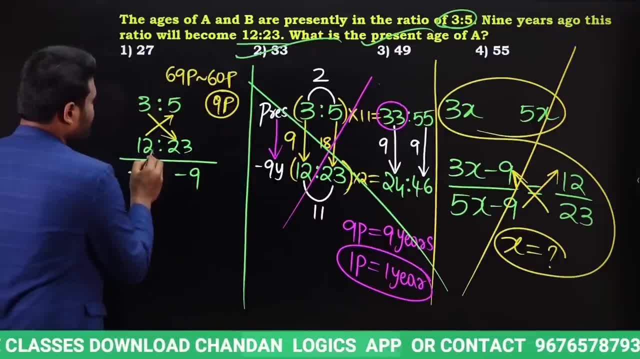 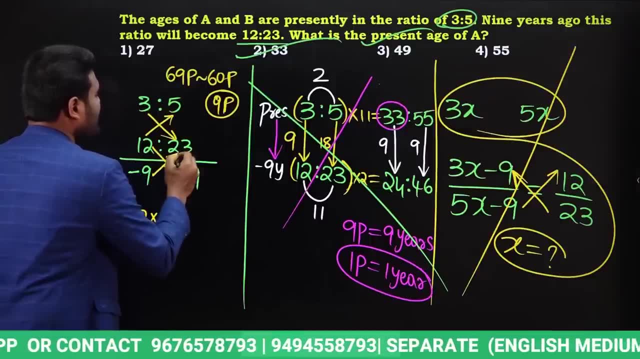 So difference in terms of parts is 9 parts. Similarly, 12 into minus 9.. Now, this is nothing but minus 9 into 12.. Okay, Similarly, minus 9 into 23.. Minus 9 into 23.. Minus 9 into 23.. And 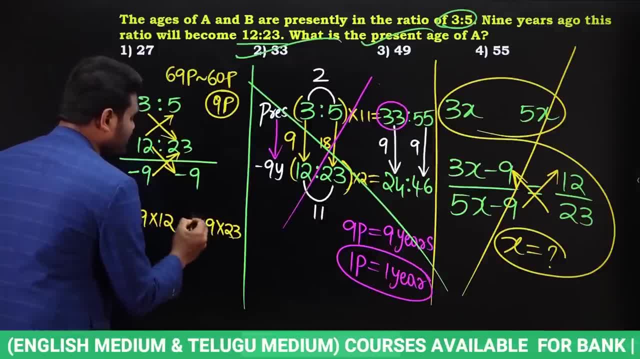 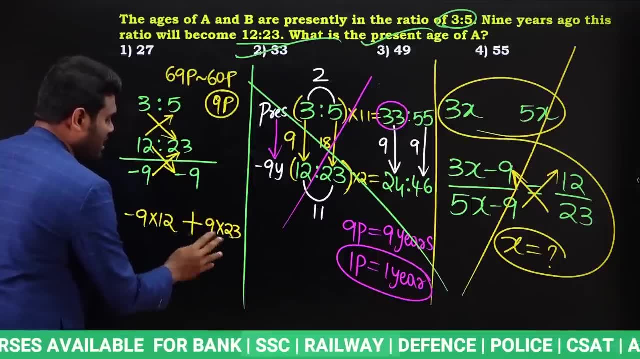 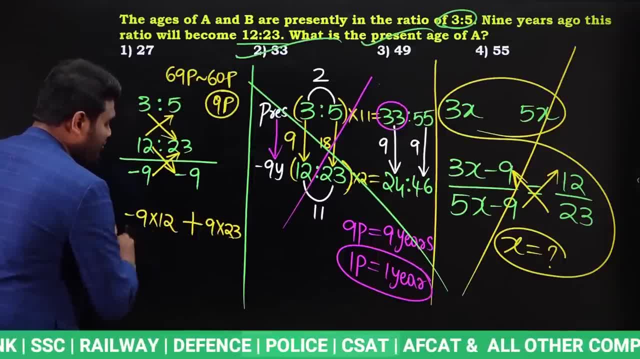 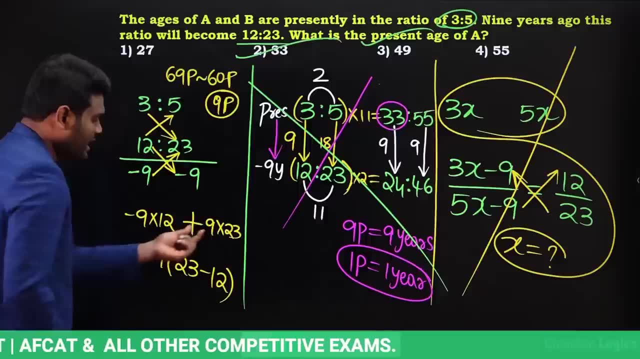 am going to do is I am going to take 9 common. If I take 9 common, this is going to be how much 9 common? Then it is going to be 23 minus 12.. Yes or no? If I take 9 common, this is 9 into 23.. 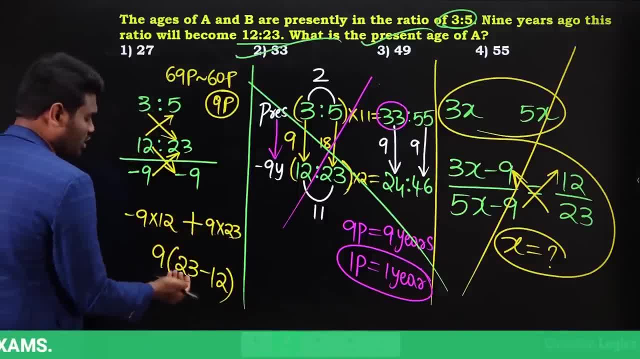 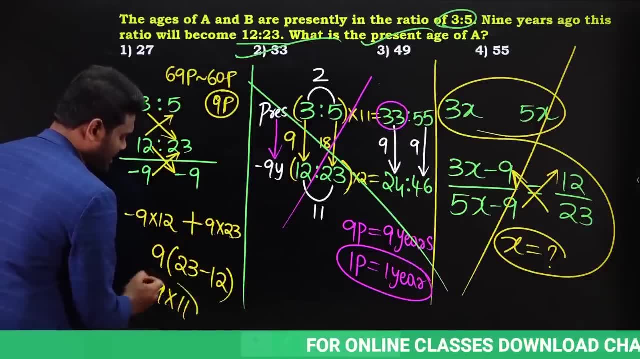 9 into 23 minus 9 into 12.. You can write in this way, Yes or no. 9 into 23, minus 9 into 12.. If you take 9 common, it will be 23 minus 12, which means 9 into 11.. Now observe: here We got in terms of: 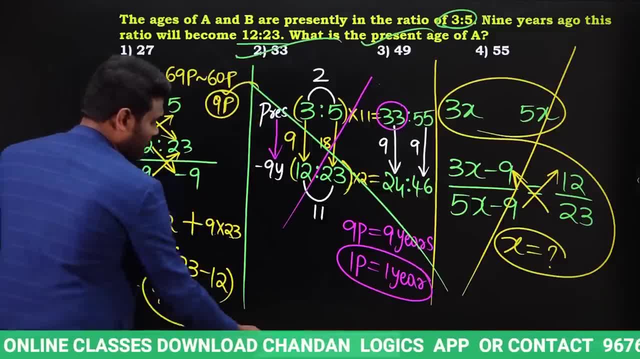 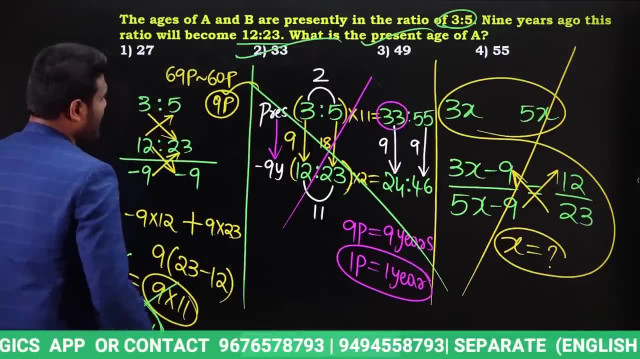 parts 9 parts 9 parts equal to 9 into 11.. Now, from this, if you observe 9,, 9 gets cancelled, So we can say 1 part equal to 11.. If 1 part is 11, now we need to know the present age of A Present age. 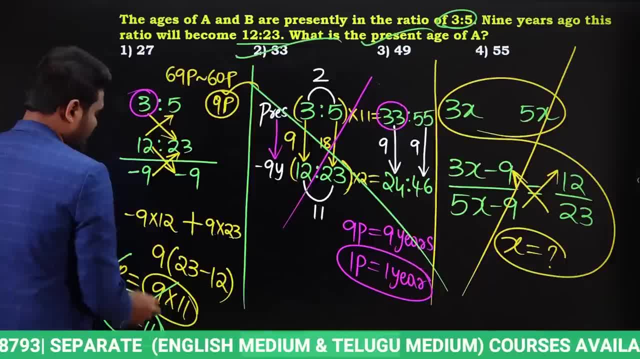 of A is going to be? how many parts? Present age of A is 3 parts. If 1 part is 11, 3 parts will be 3 into 11.. That is going to be 33.. Yes, Now, even this is going to be 3 into 11.. That is going to be. 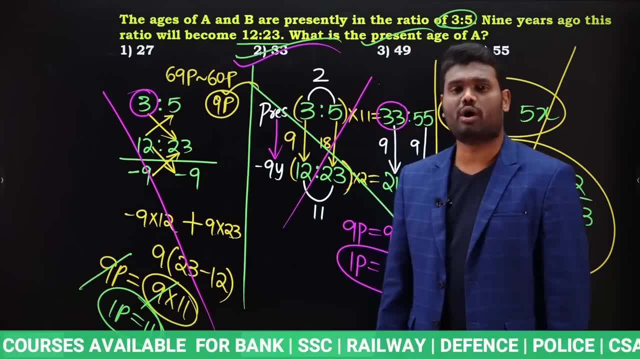 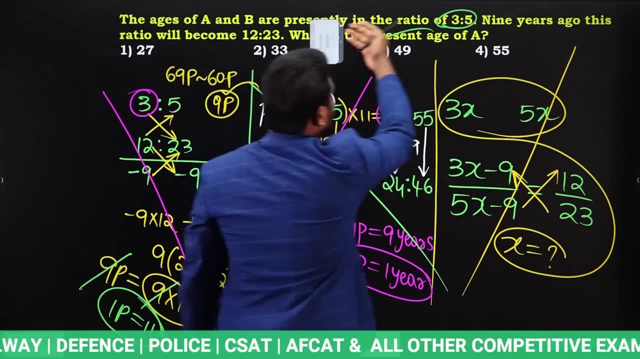 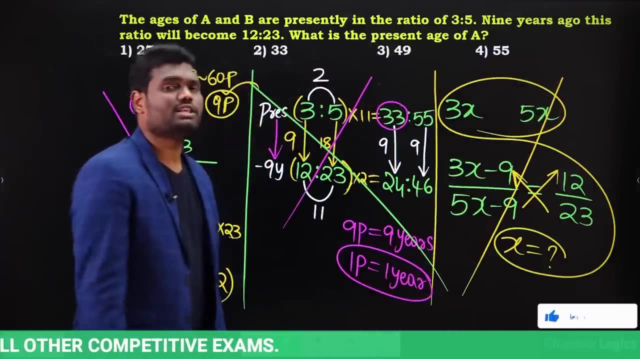 3 into 11.. This is going to consume lot of time in examination. Then, how to solve these type of questions very easily in examination? Observe carefully What you can do is whenever you have questions based upon ages, what you can do is, most of the time, 95% of time- you can solve these. 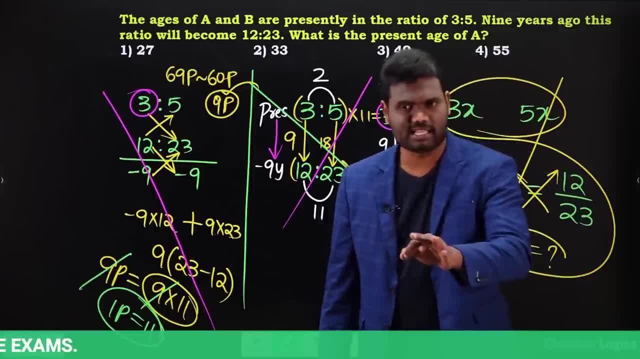 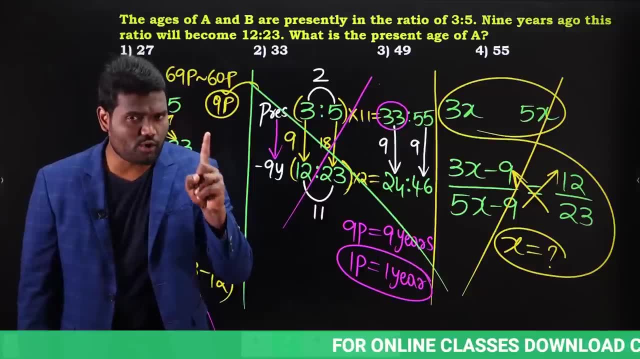 questions. just by using option verification? Yes, Just by applying option verification you can solve these questions. But when you are applying option verification, you have to read the question carefully, understand the question carefully and then you can solve the question. So this is going. 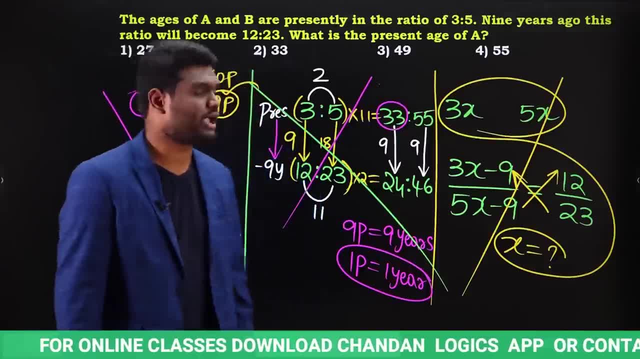 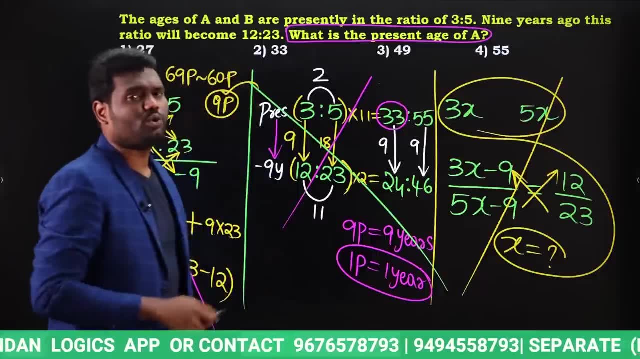 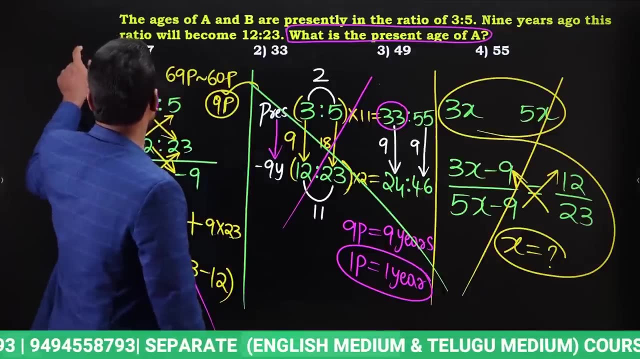 carefully and then you have to apply option verification. Okay, Now our requirement. what is our requirement? Our requirement is present: age of A. Whenever you are trying to apply option verification, first of all you need to know what are the given options. So, given options are present. 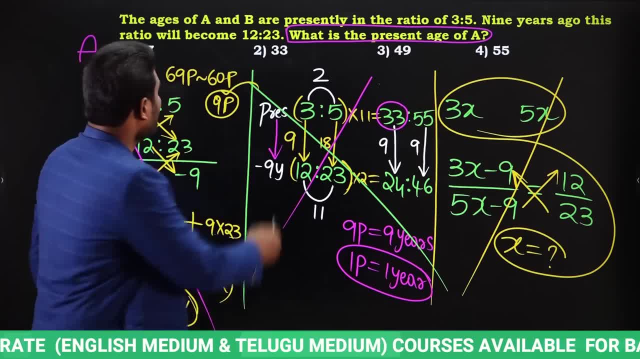 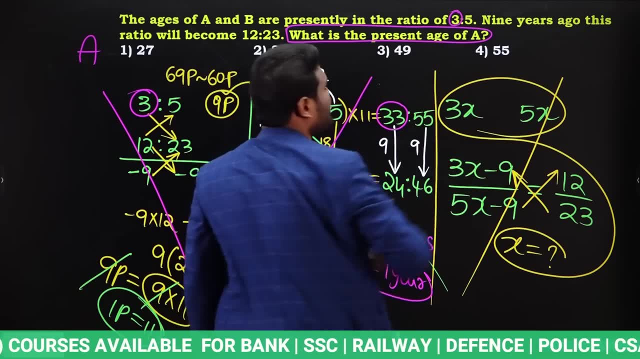 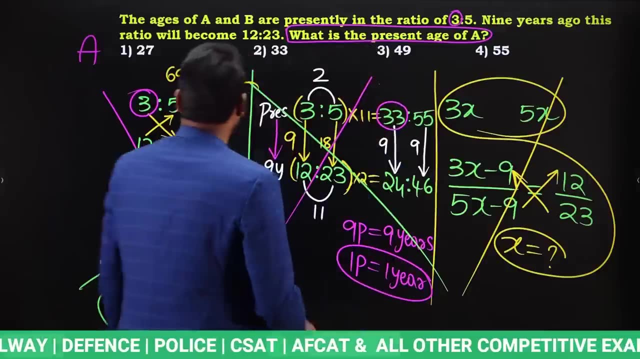 age of A. Okay, These are present age of A. In the question it is very clearly said that AB present ratio is 3 ratio 5, which means A's present age is going to be 3 multiple. 3 ratio 5 means 3 into something. 3 into something means 3 multiple. Yes or no? Now? 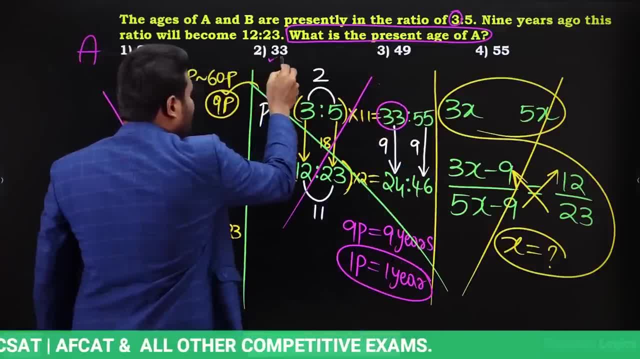 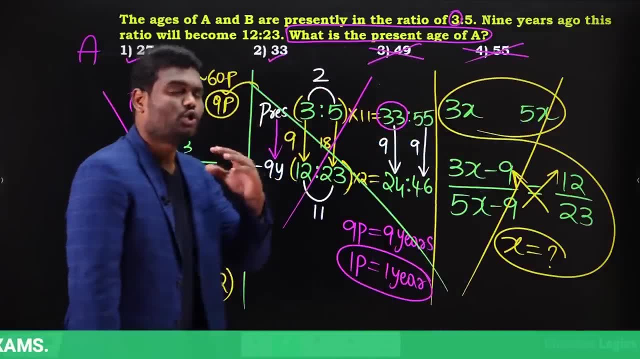 is 27 multiple of 3? Yes. Is 33 multiple of 3? Yes. Is 49 multiple of 3? No. Is 55 multiple of 3? No, Which means out of 4 options, 2 options eliminated. Okay, Now we have 2 more options. You need not. 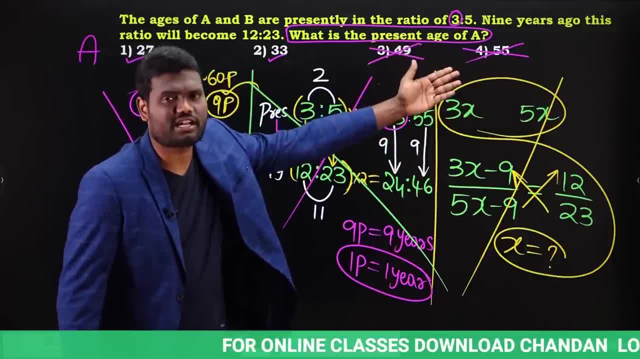 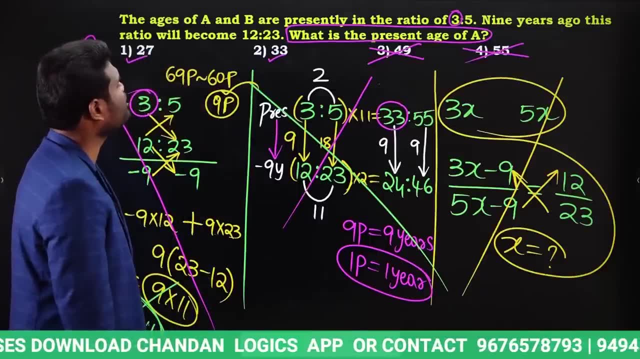 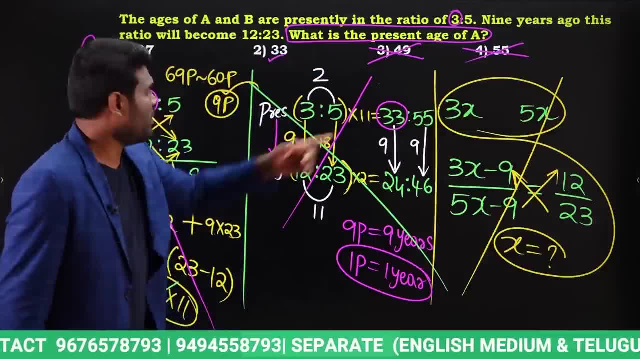 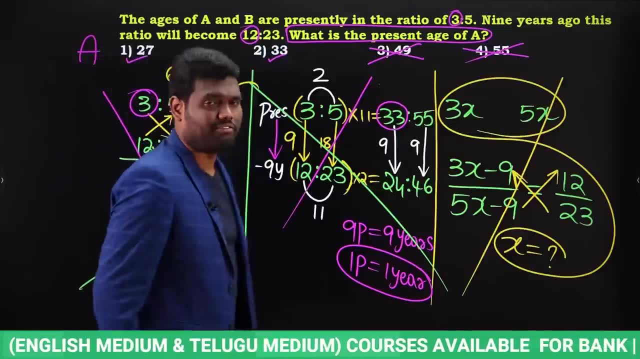 back ratio: 12 ratio 23.. I am looking for A, Why means in options. I have A As I have A. that is reason now A's age should be multiple of 12.. A's age should be multiple of 12 when 9 years back. 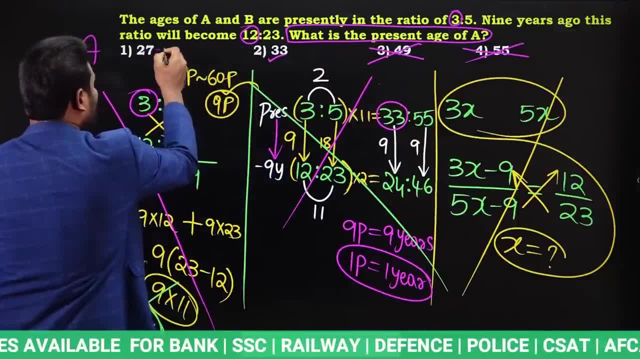 9 years back. it should be multiple of 12.. 9 years back means I need to subtract 9.. Yes, From 27,. if you subtract 9,, this is going to be how much 18.. Yes, He is 18.. 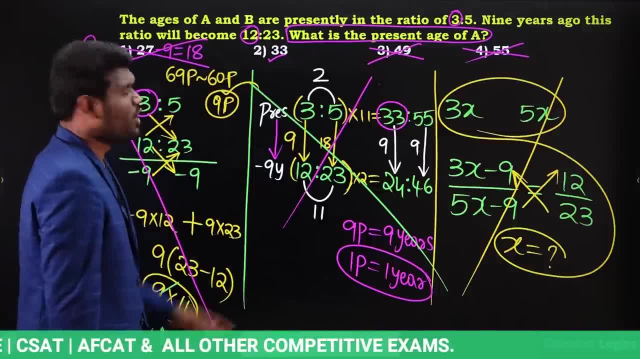 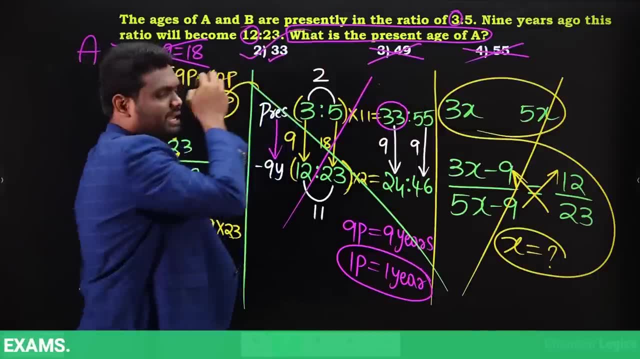 Multiple of 12?? No, So this is also going to be wrong answer. Yes, Why means 18 is not multiple of 12?? Now observe carefully: Out of 4 options, 3 options eliminated, which means definitely I can say 33 is going to be my answer: Yes, If you want, you can verify. also If you verify 9 years back. 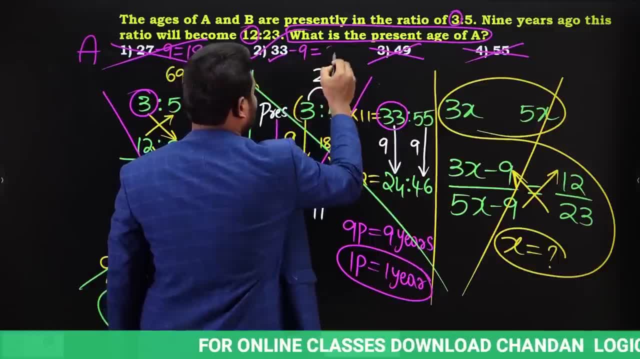 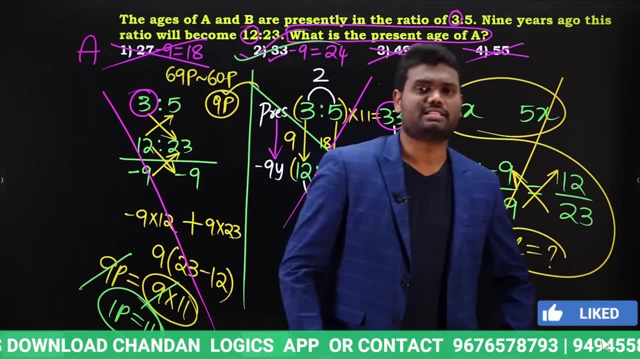 means 33 minus 9.. If you subtract 33 minus 9, it is going to be 24.. Now look, is 24 multiple of 12?? Yes, 24 is multiple of 12.. So we can say: answer is going to be 33.. So 33 is going to satisfy. 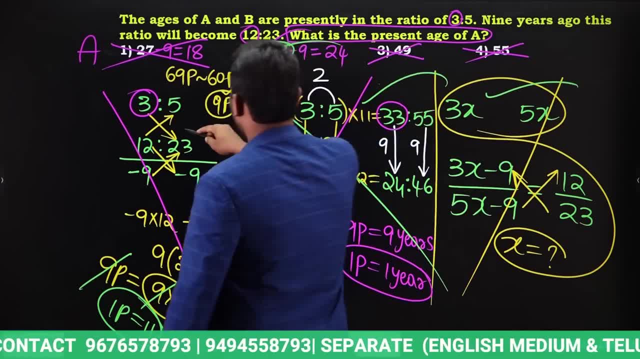 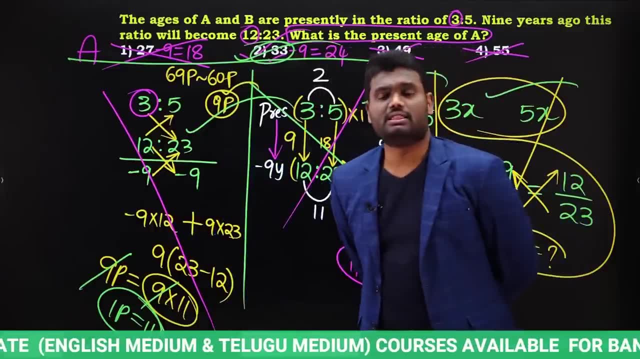 the condition. So you can solve either in this way or in this way, or in this way, or you can solve using optional verification. also, When you are trying to solve question using optional verification, this question can be solved without using pen and paper. But for all these techniques, 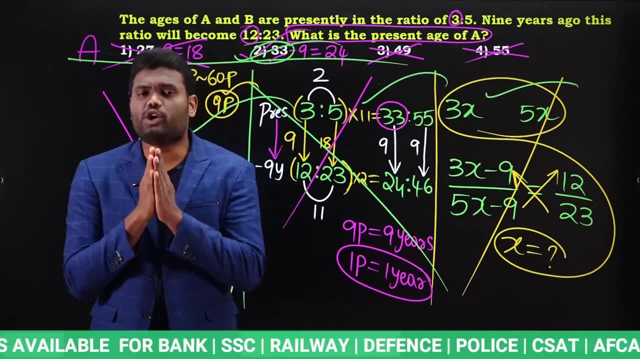 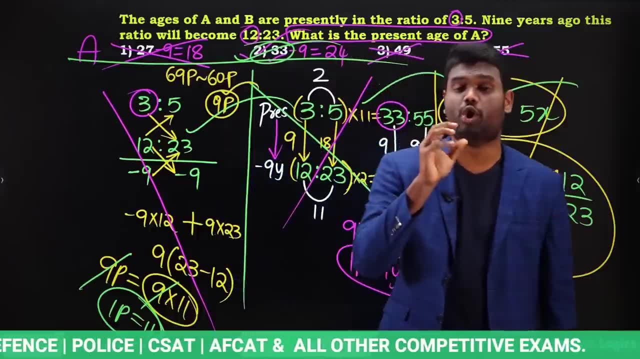 obviously you have to use pen and paper, So that is reason. try to be always smart and unique in examination. If you are smart and unique in examination then obviously you can save lot of time in examination. Just getting the mark is not important. 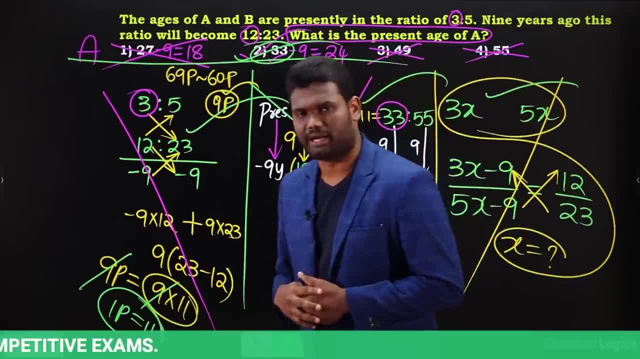 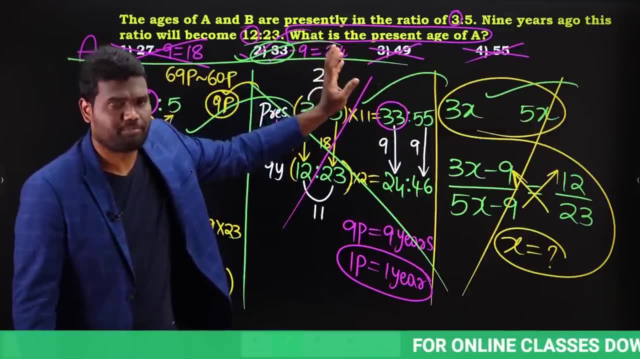 In how much time you are getting the mark. it is very, very important in competitive exams. Always you have to be smart, Always you have to be unique. Try to utilize the information given in the question properly. If you are able to utilize the information given in the question, 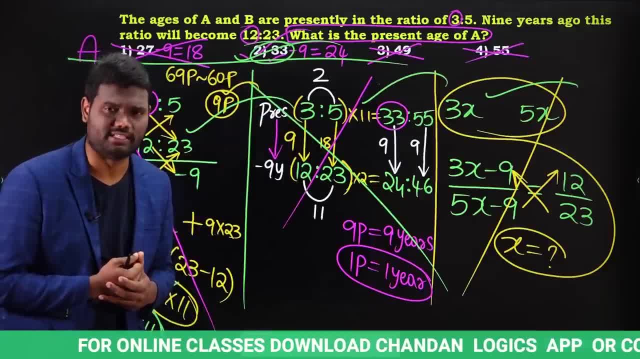 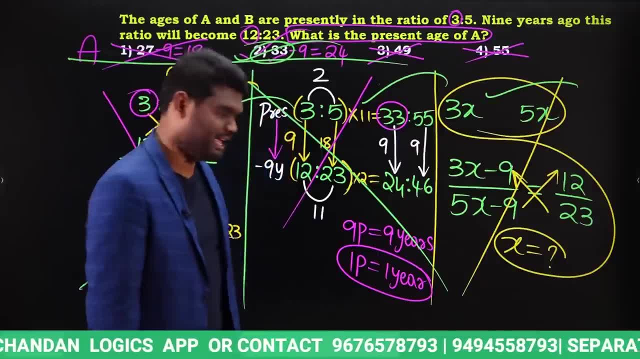 properly, then you can solve these type of questions very, very easily. Almost 95% of questions from topic ages can be solved just by using optional verification. Yes, We can solve one more question. Look at this: The respective ratio of the present age. 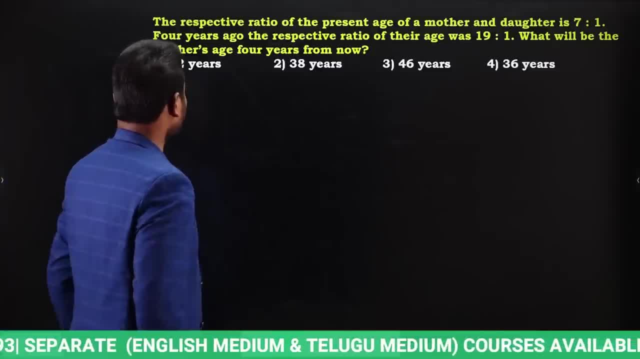 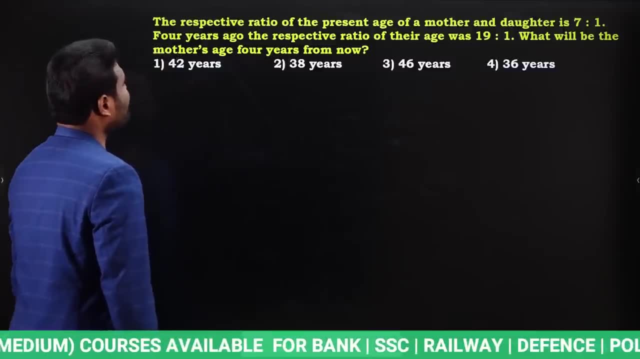 of a mother and daughter is 7 ratio 1.. 4 years ago, the respective ratio of their age was 19 ratio 1.. What will be the mother's age 4 years from now? We are supposed to know mother's age. 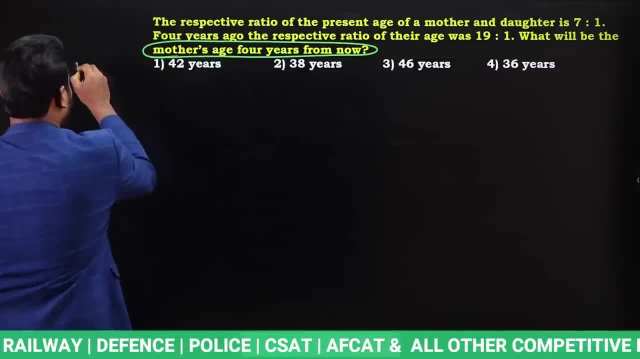 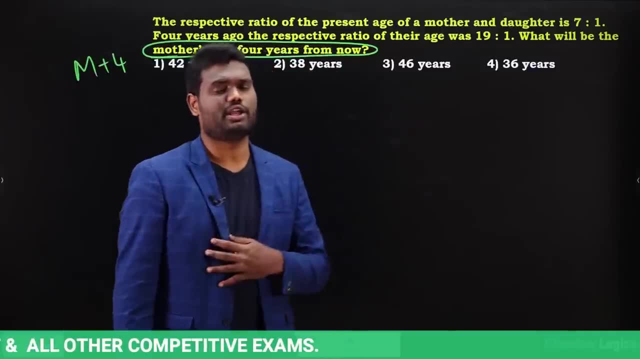 4 years from now. So given options: are mother's age after 4 years Yes or no? Mother's age after 4 years? Now, even now, this question can be done using optional verification. If you want to verify optional verification, first of all you have to know the age of the mother and daughter. If you 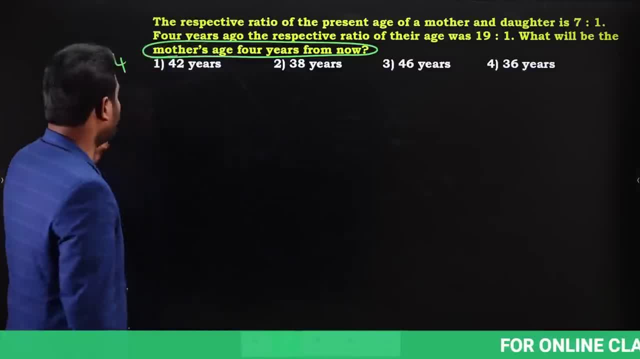 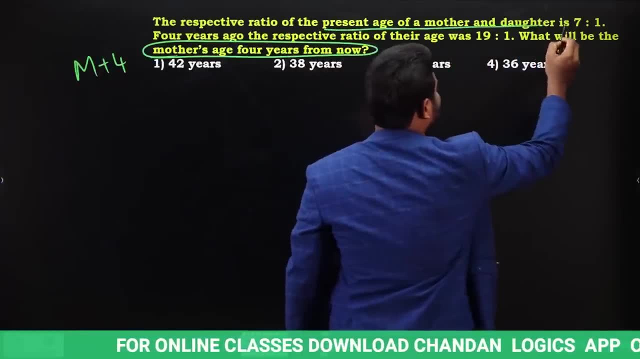 need to know what is the option. we came to know that options are nothing but mother's age after 4 years. Now what is given in the question? In the question it is said present age of mother- daughter is 7 ratio 1., Which means present age of mother should be multiple of 7.. Yes, Mother's. 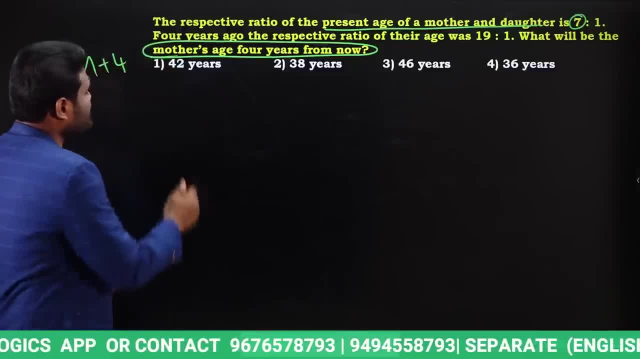 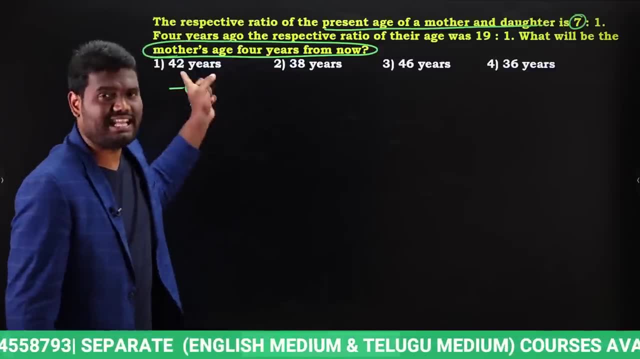 present age should be multiple of 7.. If I need to know mother's present age means I need to subtract 4.. Why means These ages are after 4 years? After 4 years, these are ages of mother. If I need to know present age of mother, I need to subtract 4.. Why means These ages are after 4 years? 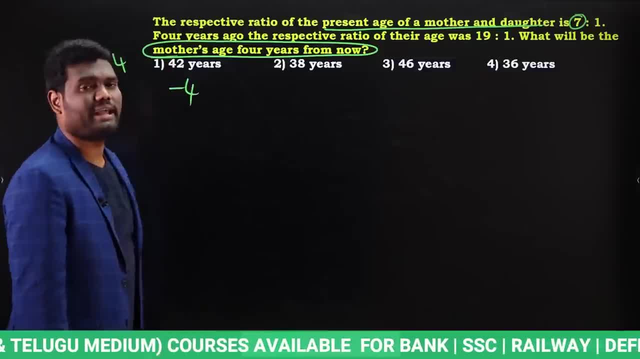 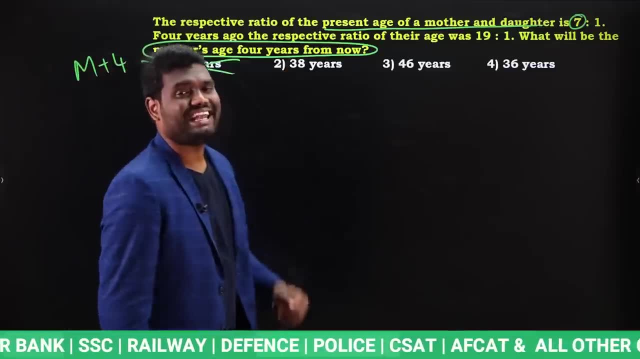 So present age means I have to subtract 4.. Now subtract 42 minus 4, it is going to be 38. Is 38 multiple of 7?? No, So this is wrong answer. Next, 38 minus 4, that is going to be 34.. Is 34 multiple? 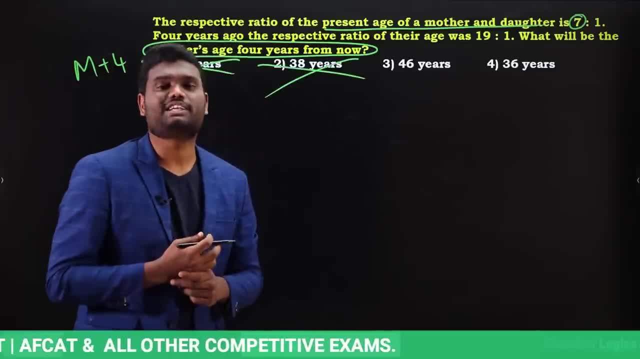 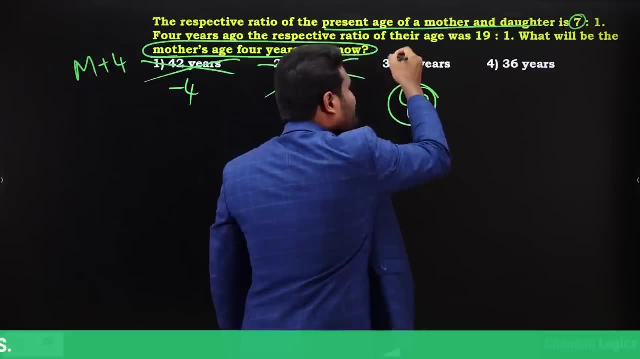 of 7?? No, Wrong answer. Next, 46 minus 4, it is going to be 42.. Yes, Is 42 multiple of 7?? Yes, 42 is multiple of 7.. So this can be our answer. Next, 36 minus 4, it is going to be 42. Yes, So. 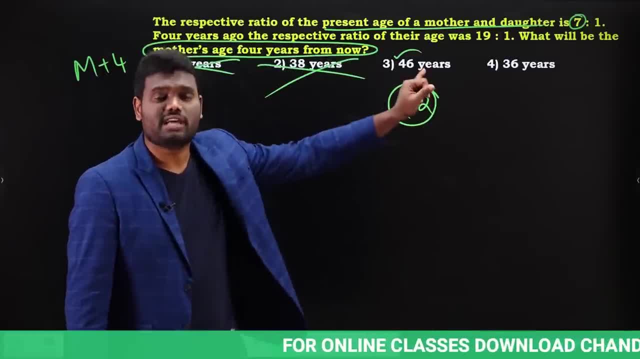 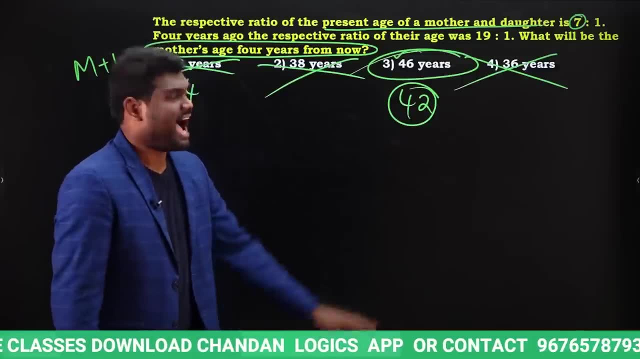 36 minus 4, it is going to be 32.. Yes, Now is 32 multiple of 7?? No, So this is wrong answer. So I can simply say: answer for this question is going to be 46.. And look here, these are the exact. 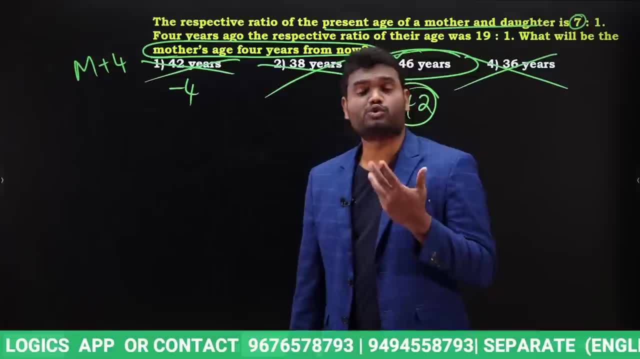 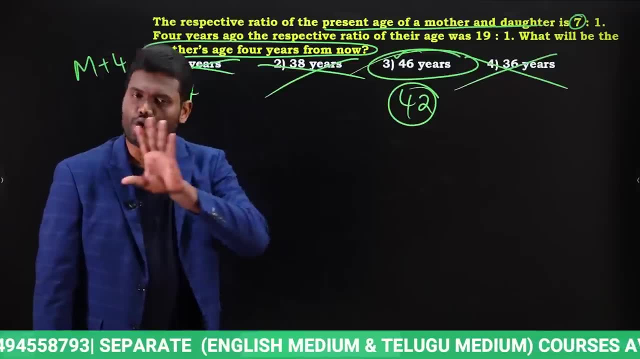 questions: exact options that came in examination. Now, so many students, they will think like options are framed in such a manner where it is going to be a multiple. No, it is not framed by me. These are the exact questions that came in examination. If you want, even you can try. 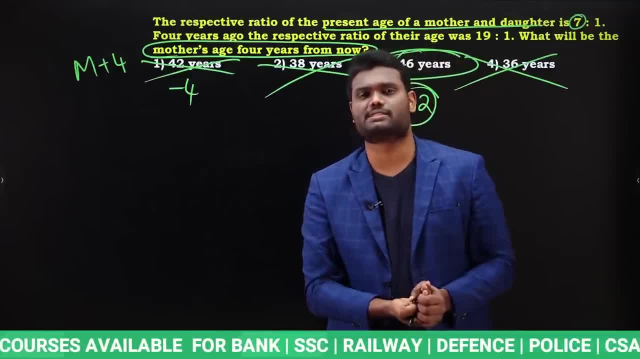 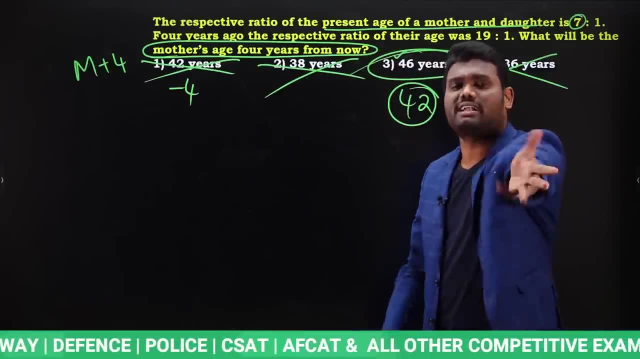 you can open the book If you want, you can open the book. If you want, you can open the book And you can try questions. whatever that came in ages. 95% of questions definitely you can solve just by looking at the question itself. Yes, it is true. If you want, you can try it. 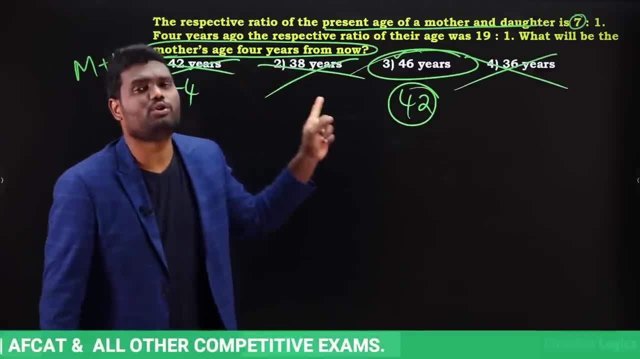 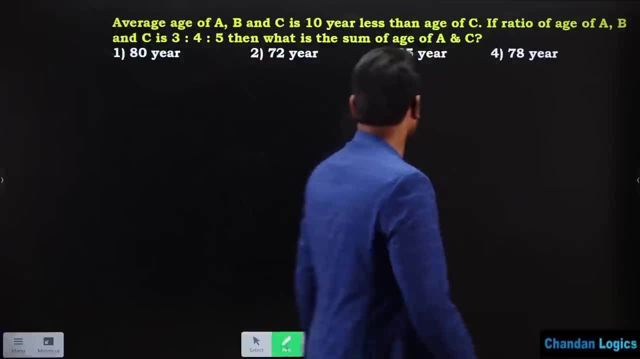 Is it clear? You can try it. then you will come to know whether you are able to solve these questions without using your pen and paper or not. Okay, So answer for this question is nothing but 46 years, Very, very simple. Let us look at one more question And one more important thing. 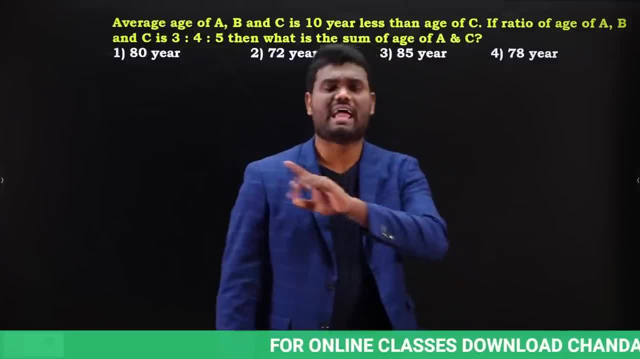 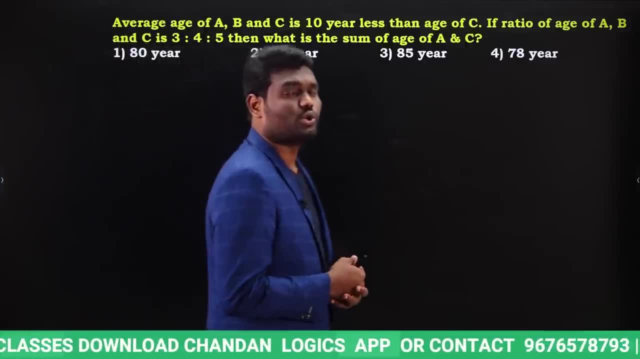 if you like this video, click on the like button and try to share this video with as many friends so that it will be very supportive for us and it will be very booster for us also, so that we'll be coming across with best content, which is going to be helpful for you in competitive exams. Okay, 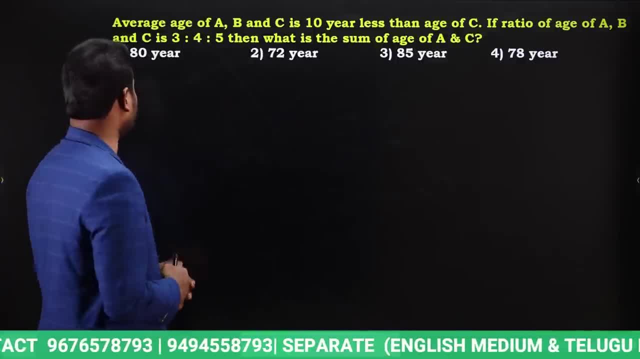 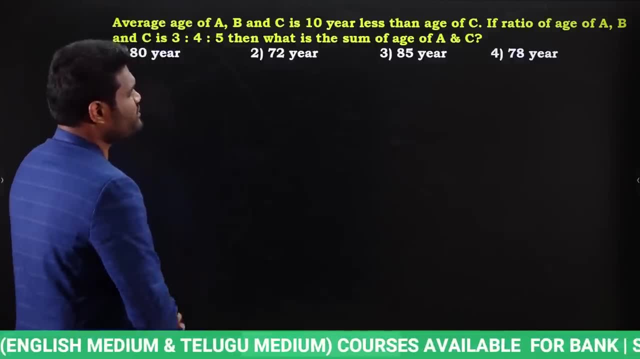 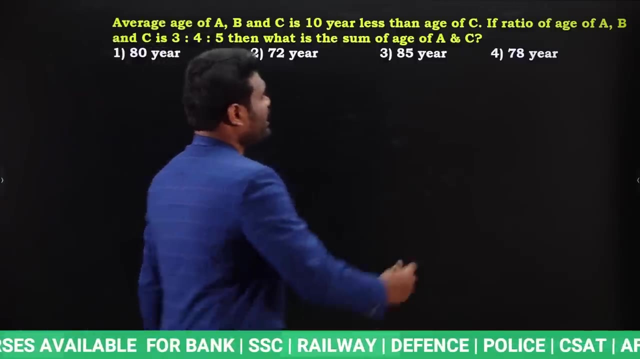 Don't forget to share with all your friends who are preparing for competitive exams. Next one: average age of ABC is 10 years less than age of C. If ratio of age of ABC is 3 ratio, 4 ratio, 5. Look here here: ratio of: 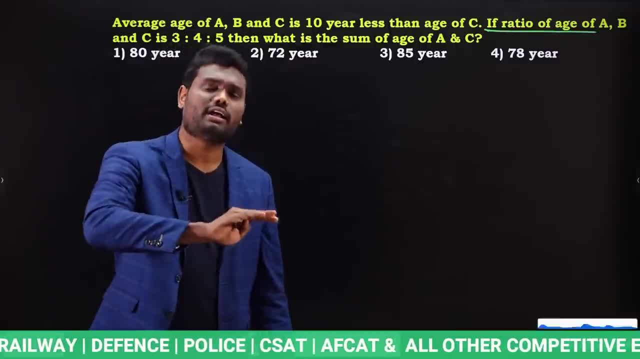 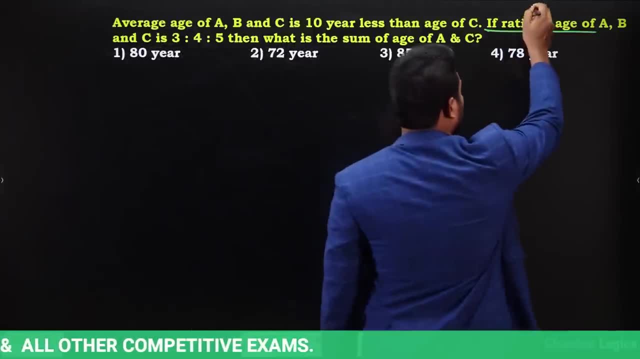 age. it was mentioned, But whether it is present age or whether it is after 5 years or whether it is 3 years ago, nothing was mentioned. If nothing was mentioned, you are supposed to take it as present age only. Is that clear, Very important point? If nothing was mentioned, you are supposed 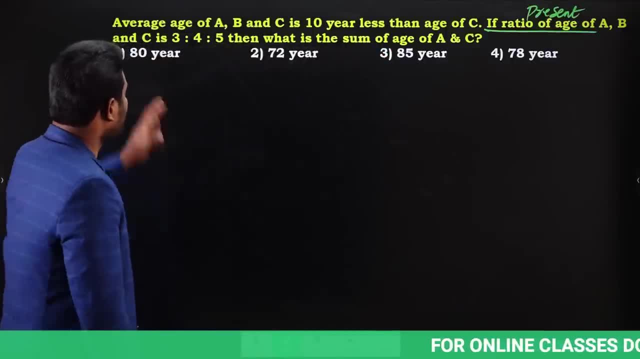 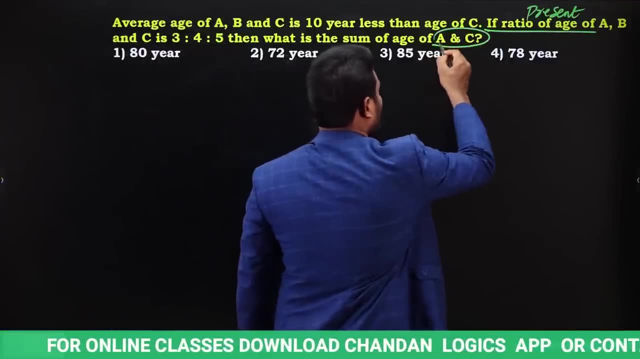 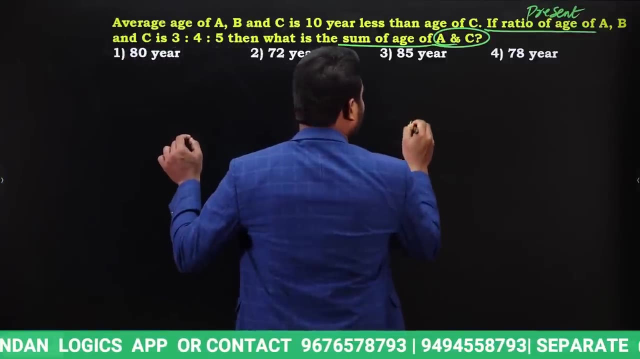 to take present age only. Present age ratio of ABC is 3 ratio, 4 ratio, 5.. We are supposed to know what is the sum of age of A and C. So we are supposed to know sum of ages of A- C, Sum of ages of A- C. Now observe carefully: In the question ABC age ratio was mentioned. Yes, 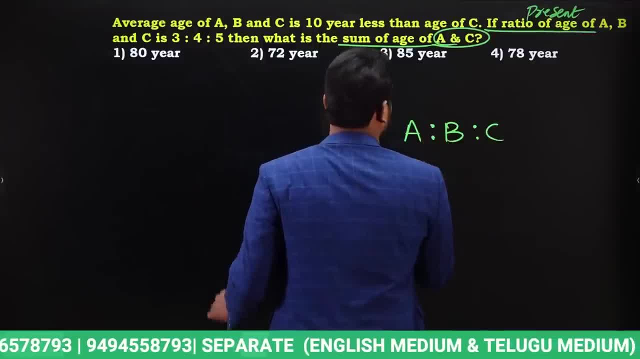 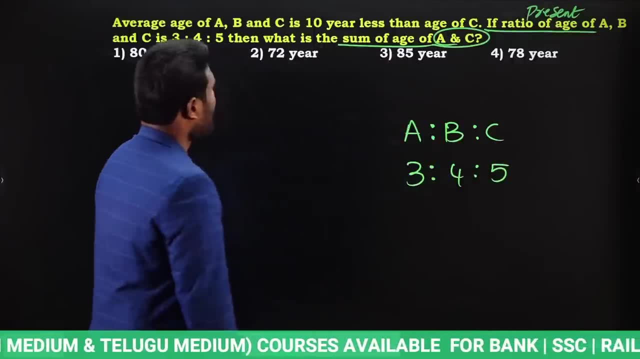 What is ABC age ratio? ABC age ratio is 3 ratio, 4 ratio, 5. Yes or no? 3 ratio, 4 ratio, 5. We are supposed to find sum of ages of A- C, which means sum of present age of A- C. Nothing was. 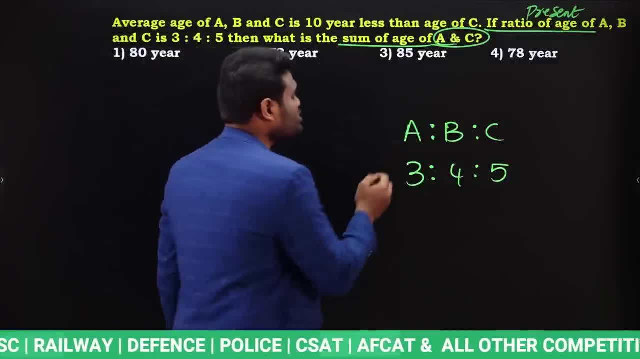 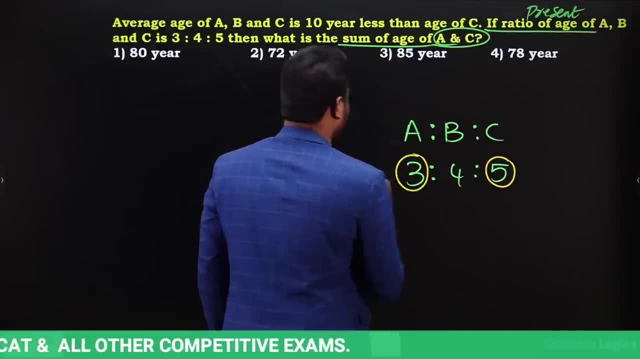 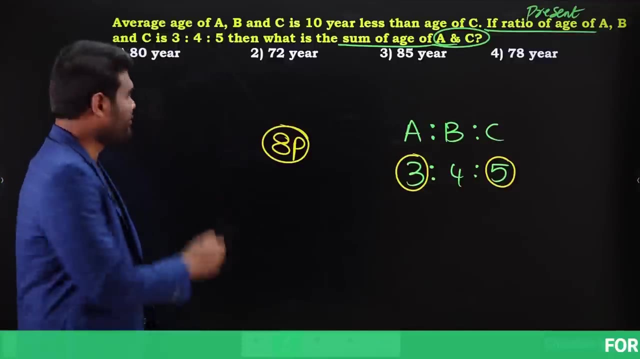 mentioned means present age. Now observe it carefully. Present age of A should be multiple of 3.. Present age of C should be multiple of 5.. Sum means 3 plus 5. That is going to be 8 parts. 8 parts means our answer should be multiple of 8.. Yes or no? Our answer should be multiple of 8.. 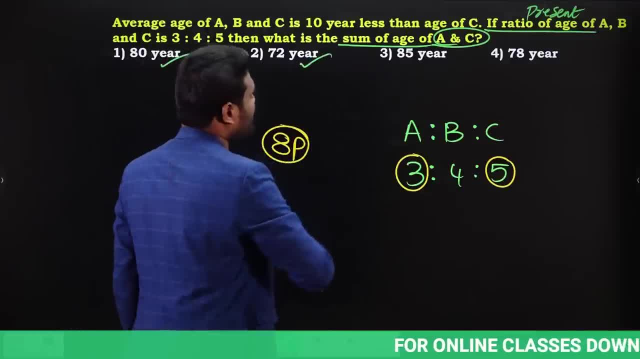 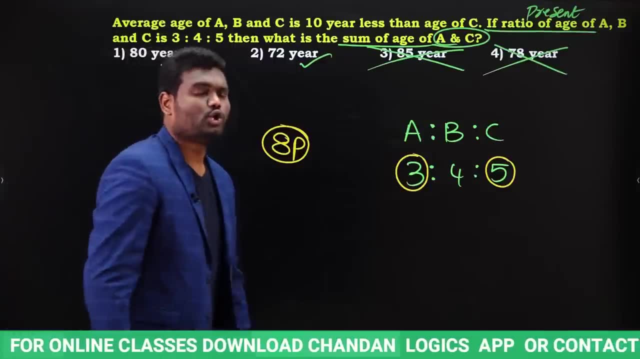 Let us check: 80 is multiple of 8.. 72 is multiple of 8.. 85 is not multiple of 8.. 78 is not multiple of 8, which means, out of 4 options, 2 options are eliminated and we are left with 2 more options. 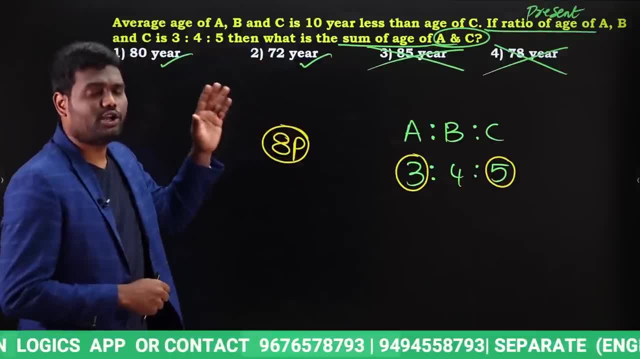 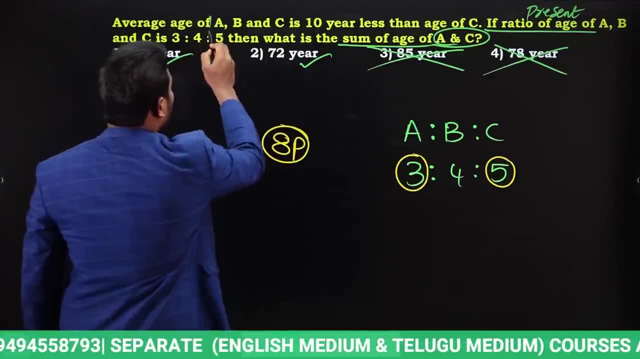 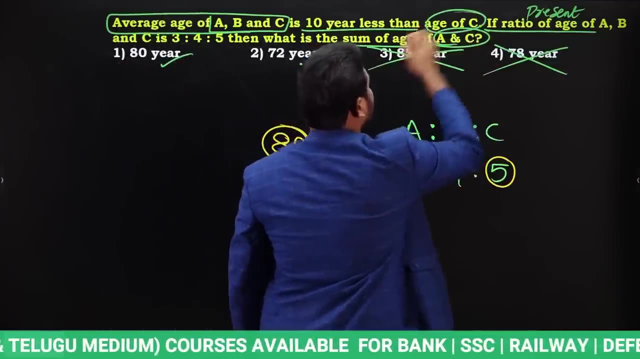 Yes, Now read the information. whatever that you have. I guess, try in the question. We have some more information. If you observe in the question it is clearly said average age of A, B, C. Average age of A- B, C is 10 years less than age of C. 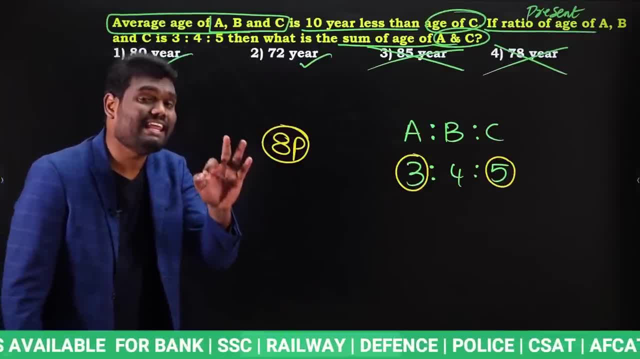 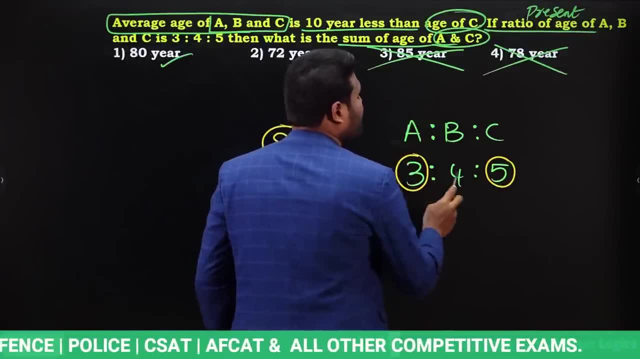 Look, average age of A, B, C is 10 years less than age of C. Now observe carefully. If you observe carefully, average age of A, B, C means 3,, 4, 5.. 3,, 4,, 5, these are nothing but ages ratio. 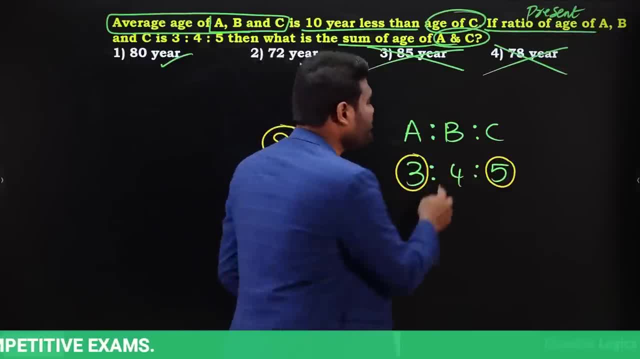 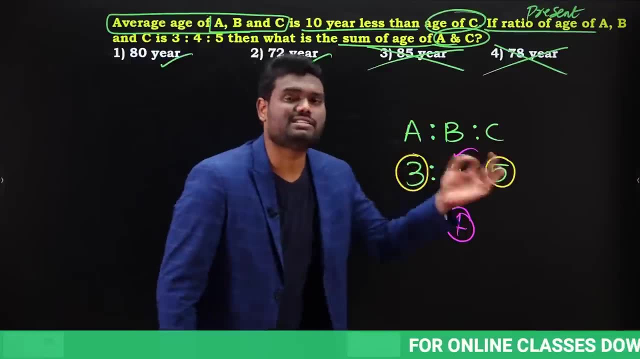 which means Average of 3,, 4, 5, is what 3, 4, 5, average is nothing but 4,, which means middle term. Y means 3,, 4, 5 are in arithmetic progression When the given series is in arithmetic progression. 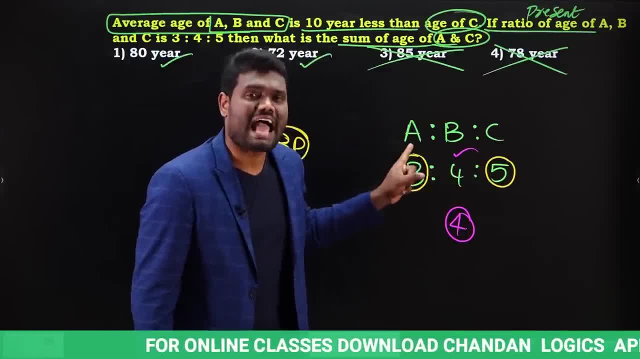 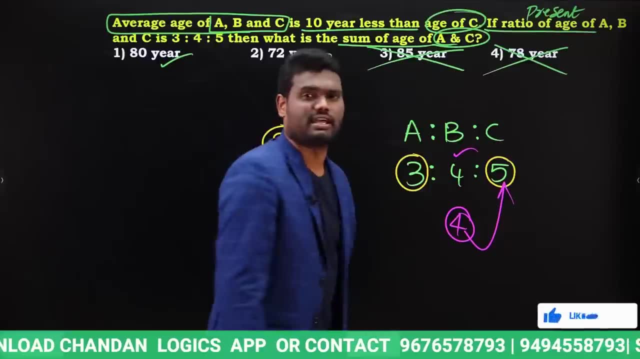 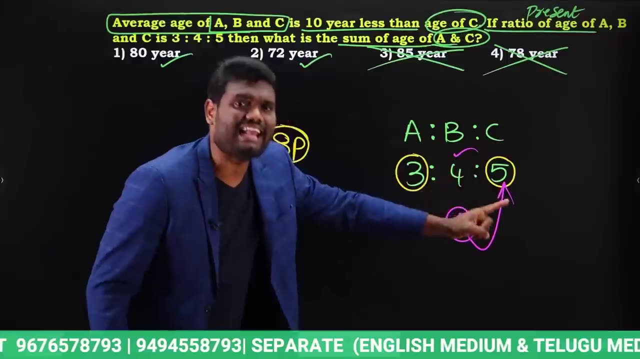 average is nothing but middle term. So middle term means 4, which means average age of A, B, C is going to be 4 parts and age of C is going to be 5 parts. And in the question it is clearly said that average age of A, B, C is 10 years, 10 years less than age of C. 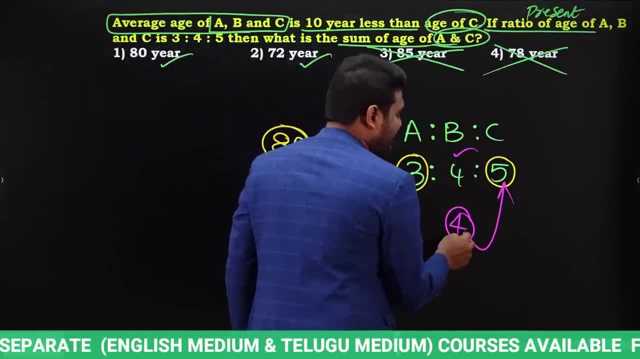 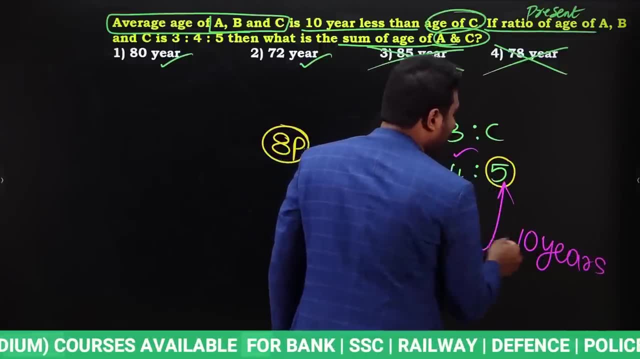 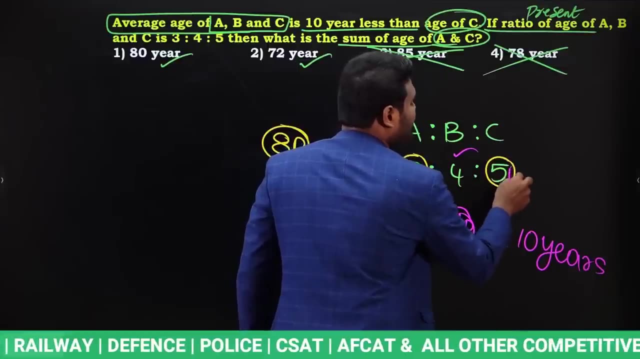 So 10 years less than age of C means difference between average and age of C is going to be 10 years, Yes or no? Now observe carefully. We know that average of A, B, C, in terms of parts, it is 4 parts. C's age, in terms of parts, 5 parts. Difference between these two is going to be: 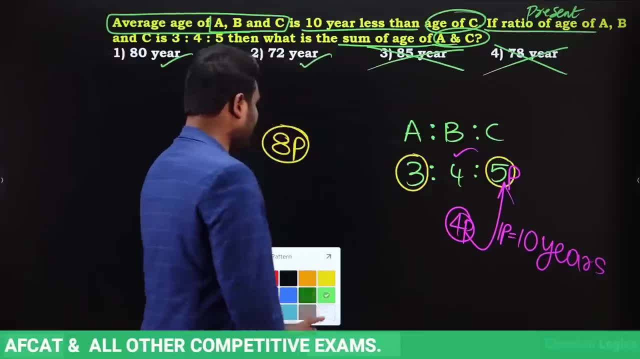 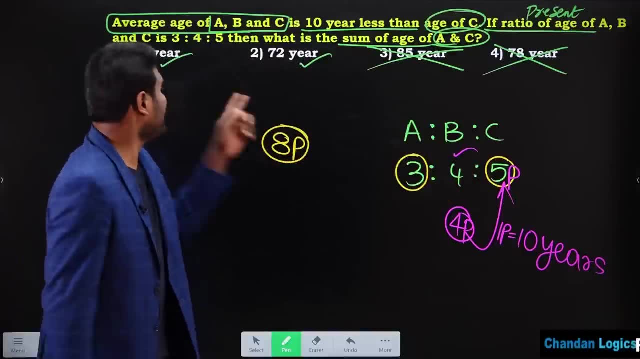 1 part. So 1 part equal to 10 years. If 1 part is 10 years we are supposed to know sum of ages of AC. Sum of age of AC is 8 parts. So 8 into 10 we can say answer is going to be 80 years, So 72 is. 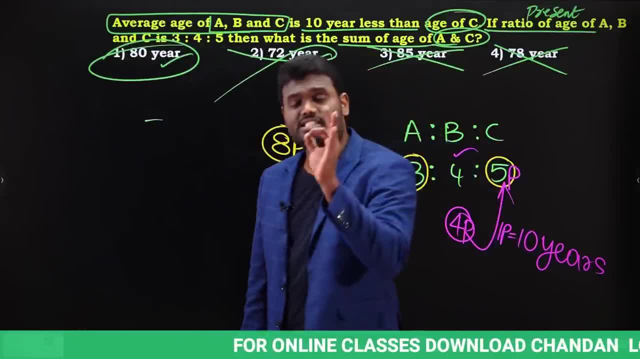 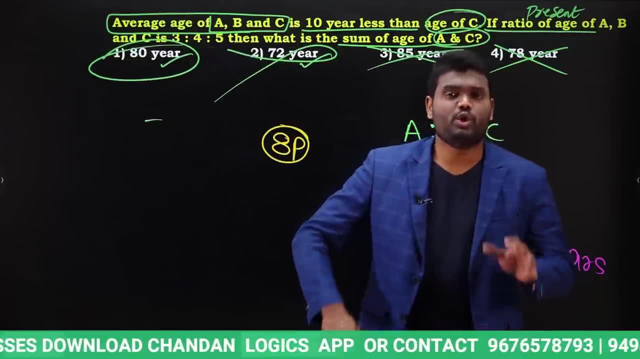 also eliminated. Is it clear? Very, very simple, Just a fraction of seconds. everything is given in the question itself and this one also exact question that came in examination. You will have complete information in the question itself, But you are supposed to be in a position to. 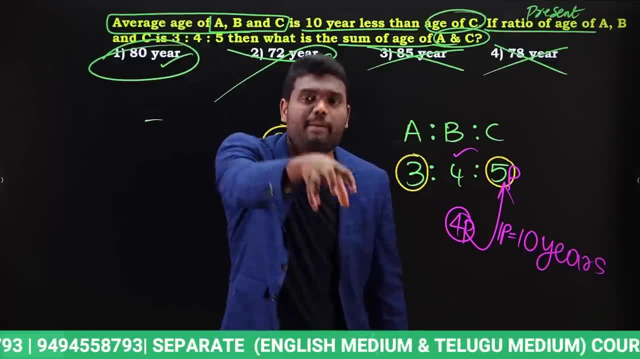 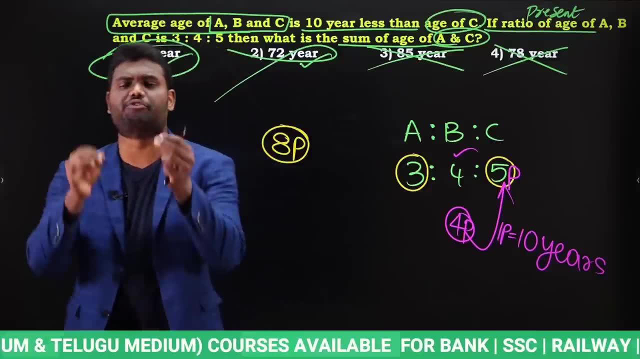 understand the question carefully and collect the key point that was mentioned in the question. If you are able to collect the key points that is mentioned in the question, then obviously you can solve these questions in fraction of seconds without using your pen and paper. Average of 3,. 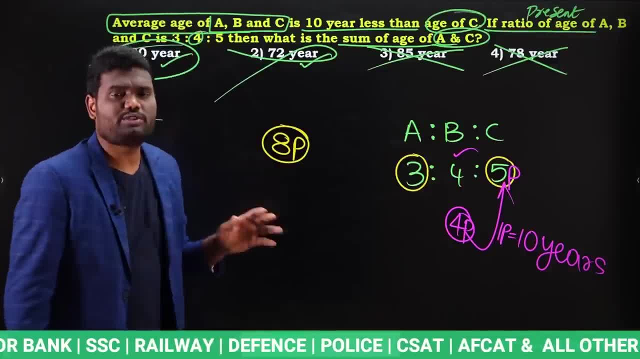 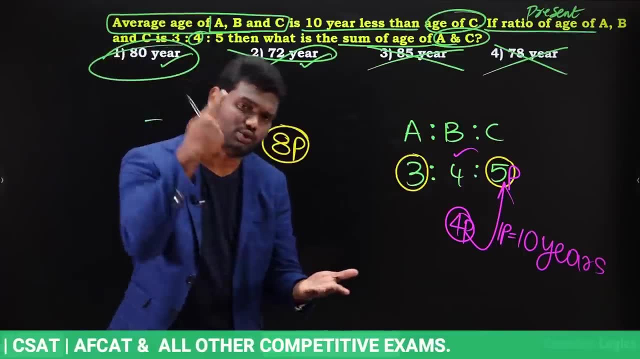 4, 5.. I can say average of 3,, 4, 5 is nothing but 4, which means average is 4 and C's age is 5 parts, 4 parts, 5 parts difference is 1 part. In the question it is clearly said that average of A 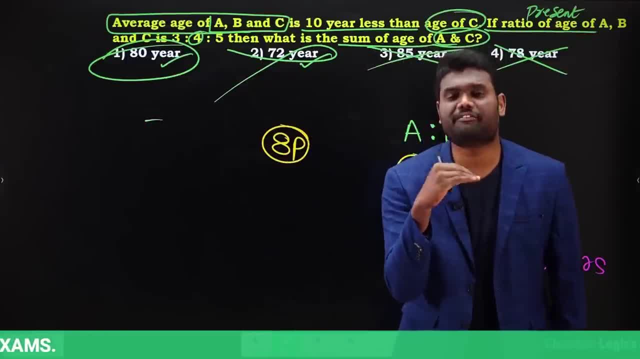 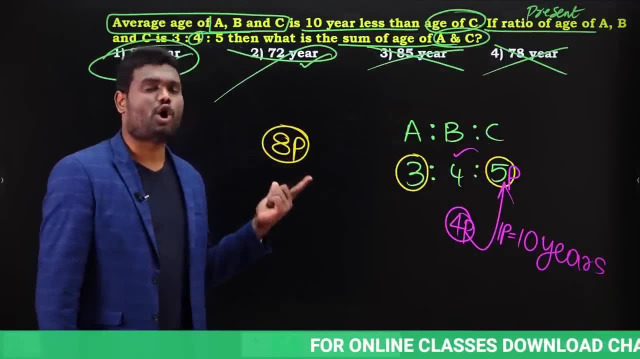 B, C is 10 years less than age of C, which means difference in terms of years is 10 years. Difference in terms of age is 10 years. Difference in terms of age is 10 years. Difference in terms of parts is 1 part. So 1 part is 10 years. We are supposed to know age of A, C together. Age of A. 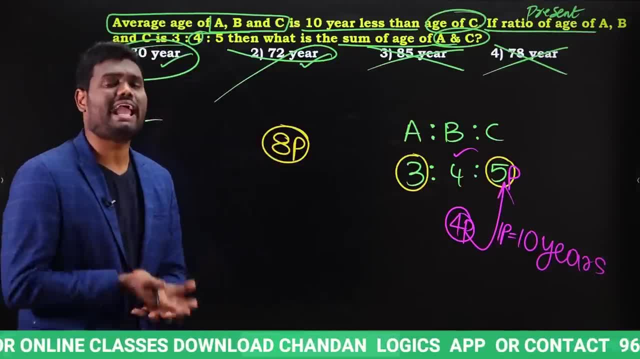 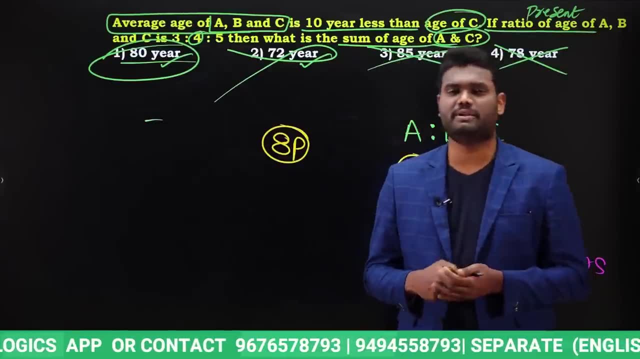 C is nothing but total 8 parts. 8 parts means 8 into 10.. 8 years, just a fraction of seconds. Always, you have to be smart and unique. You have to be smart and unique Once if you are smart and 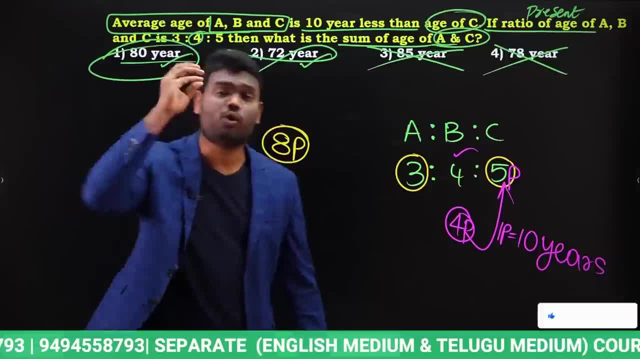 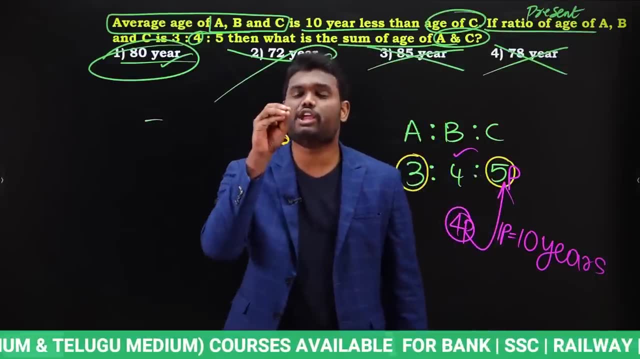 unique, then you can save lot of time in examination. When thousands, lakhs of students are writing examination, then why only you need to get the job? Just think of that. Why you need to get the job means then definitely you have to work hard, you have to be unique. 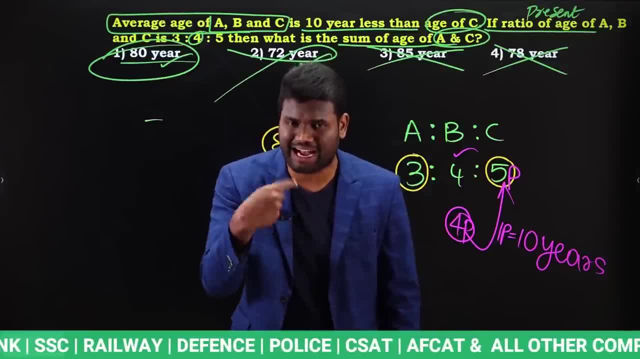 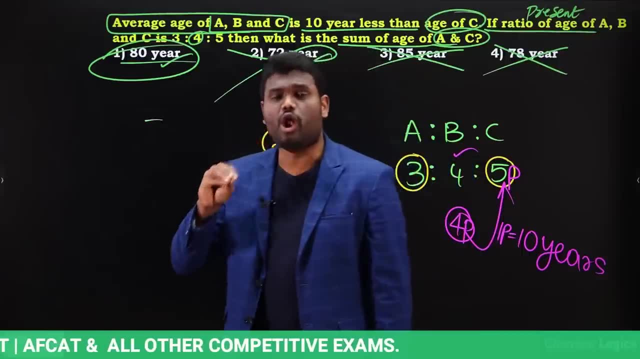 you have to be smart, you have to spend lot of time for the purpose of practice, you have to come across with many innovative thinkings, which is going to helpful for you in examination, When you are doing lot of hard work, lot of smart work. if you are going to do all of this, then 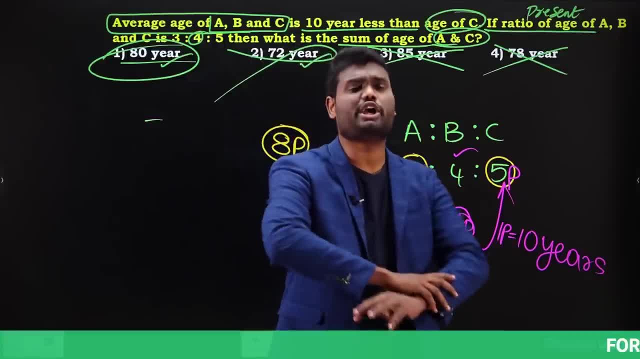 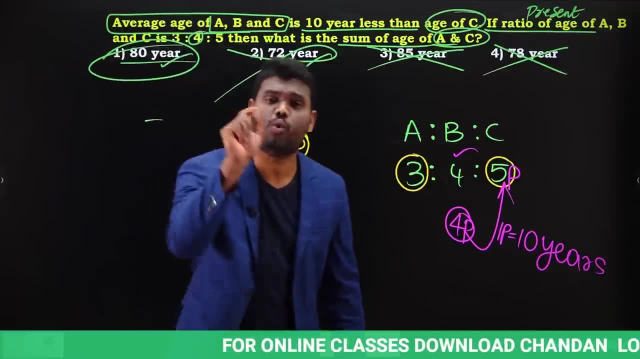 only you are going to get success. Why means we know that there is a huge competition? Any exam, whatever the examination you are going to write, there is a huge competition. In this huge competition, if you are going to be one out of those selected students means definitely your 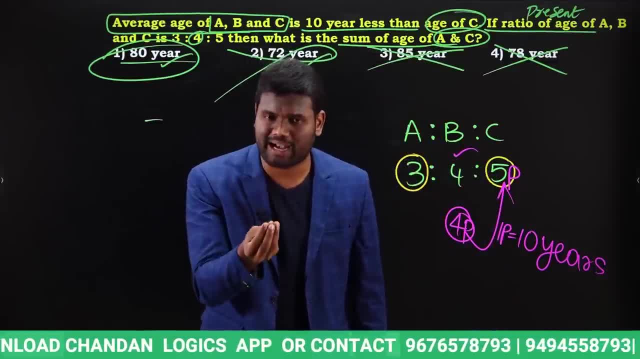 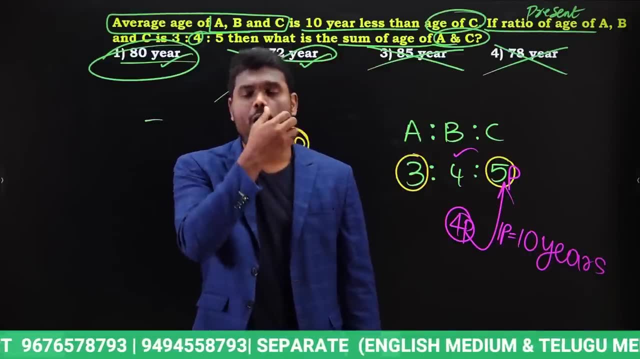 hard work, your smart work, your guidance and how well you are practicing. what are the approaches, how much time you are spending, how much time you are spending for questions, how much time you are spending every day. all these are going to play vital role. Who is going to work hard, work smart? 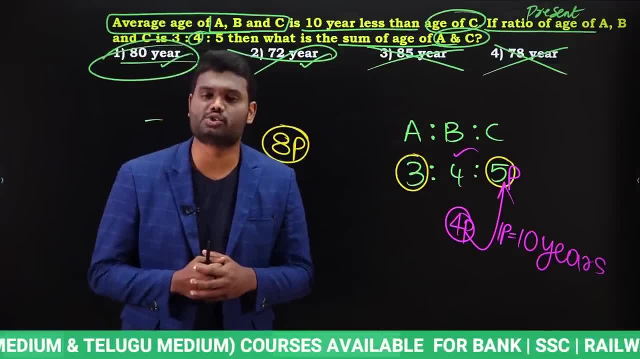 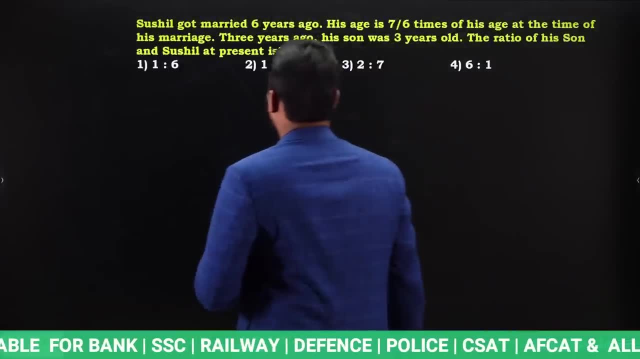 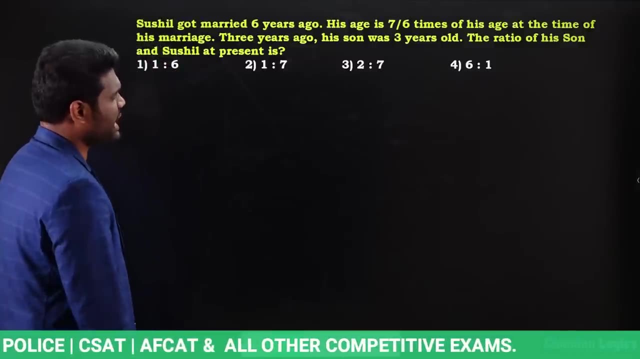 and they are going to practice regularly. only for them success is going to come in this competition. Why means there is a huge competition for competitive exams, Yes or no? Let us look at the next question. Sushil got married 6 years ago. His age is 7 by 6 times of his age at the time of his marriage. 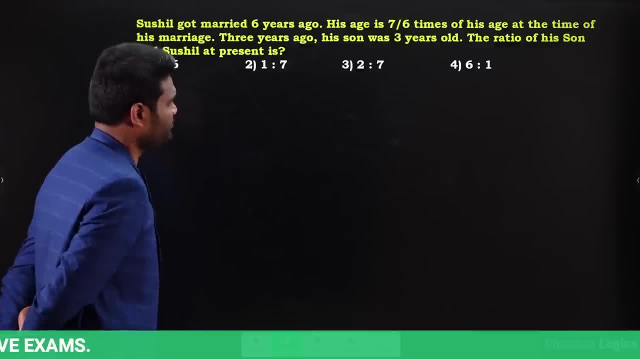 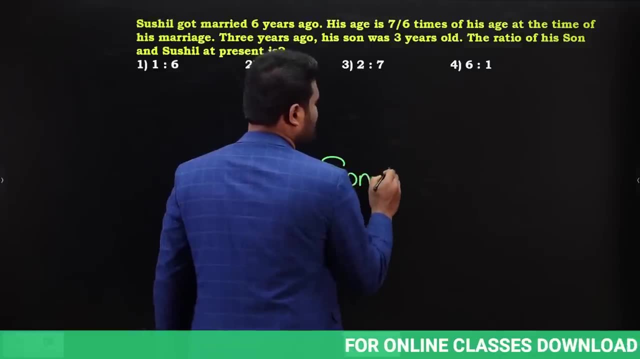 3 years ago his son was 3 years old. The ratio of his son and Sushil at present. So we are supposed to know present age ratio of Sushil's son and Sushil. So we are supposed to know Sushil's son and Sushil. 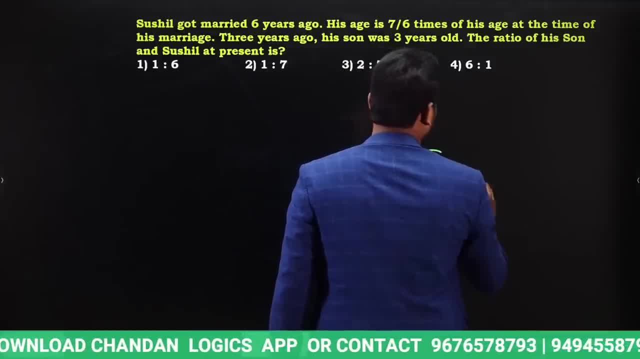 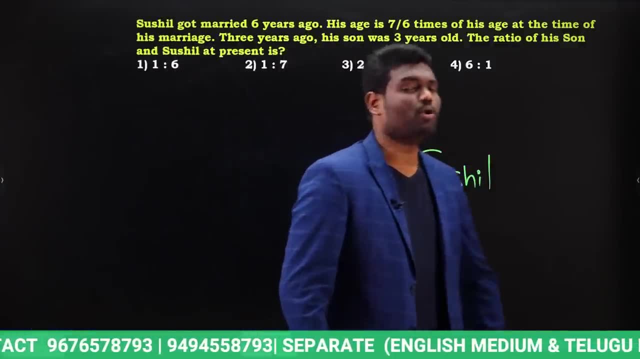 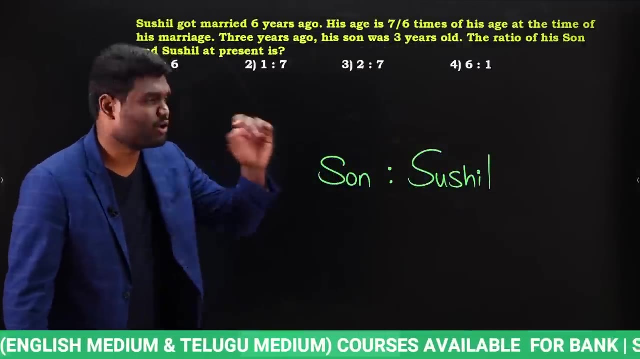 Sushil son and Sushil age ratio. This is very, very simple question. Even in this question also, complete information is given in the question itself. But most of the students they don't understand the question carefully. That is reason competitive examination, it is all about reading. 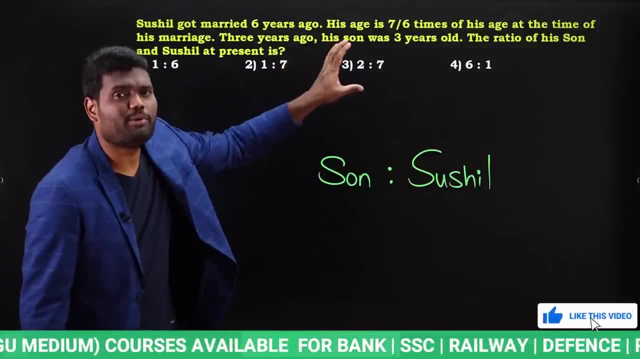 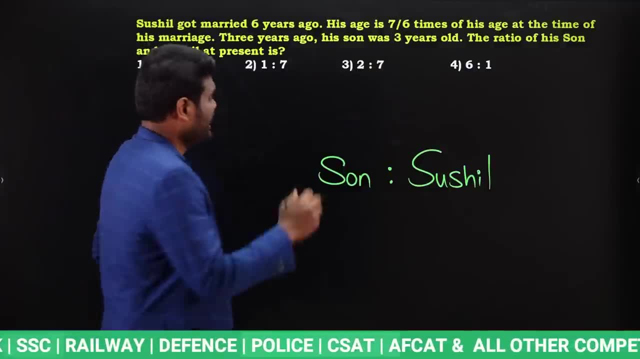 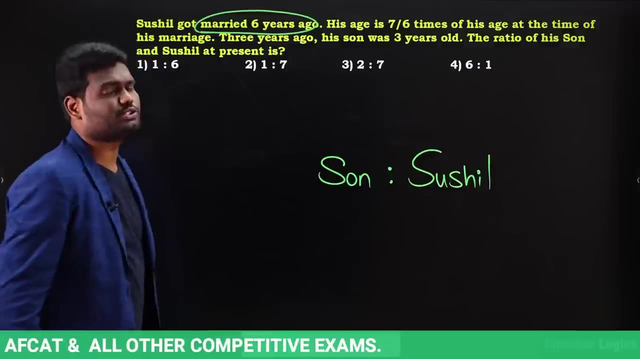 the question carefully, understanding the question carefully. Once you are able to understand question and if you are able to collect the key points, then it is very simple to mark the answer. Look here it is very clearly said: Sushil got married 6 years ago. So 6 years ago Sushil got married. His age is 7 by 6 times of 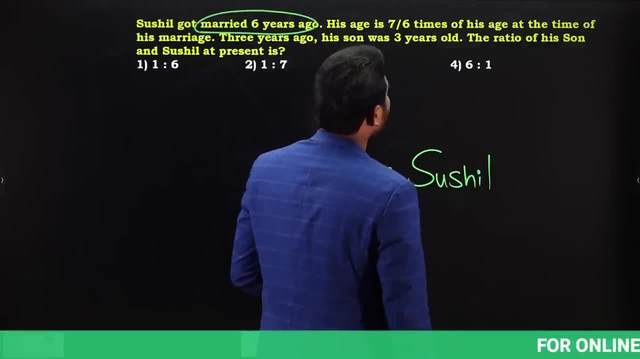 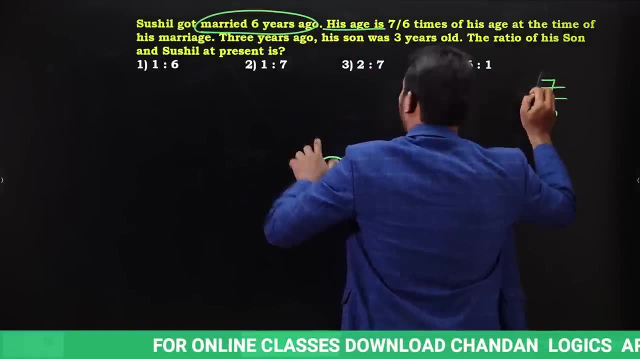 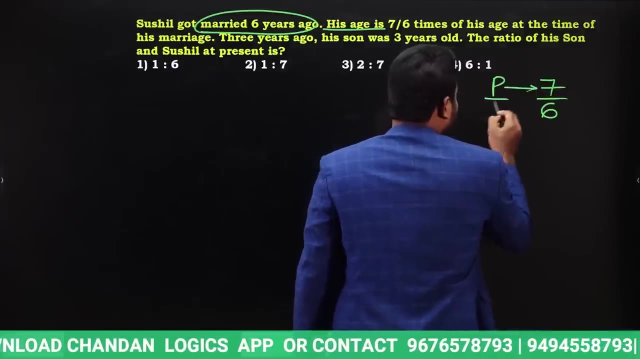 his age at the time of his marriage, Which means it is said that present age of Sushil is 7 by 6 times of his age at the time of marriage, Which means this is present age, Yes or no? This is present age and this is at the time of marriage. So Sushil got married 6 years ago. So 6 years ago. 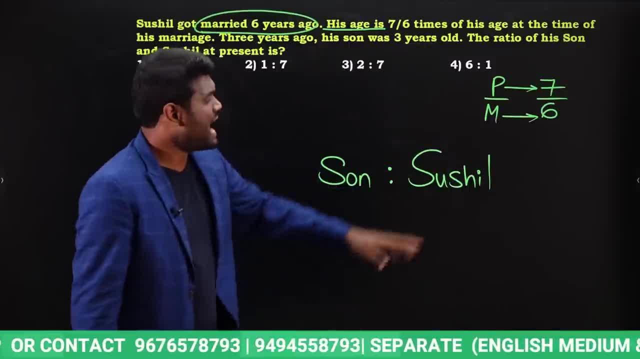 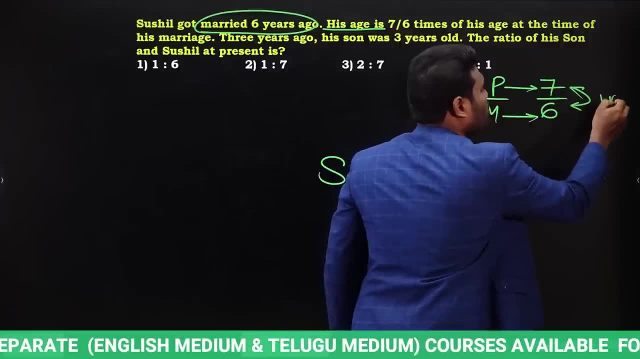 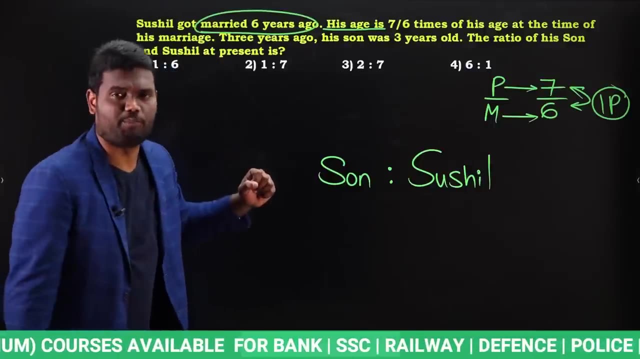 marriage percentage of Sushil is 7 parts and age of Sushil at the time of marriage is 6 parts. Now difference between these two is going to be how many parts? One part, yes or no? Difference between these two is one part and it's very clear that Sushil got married 6 years ago, which means 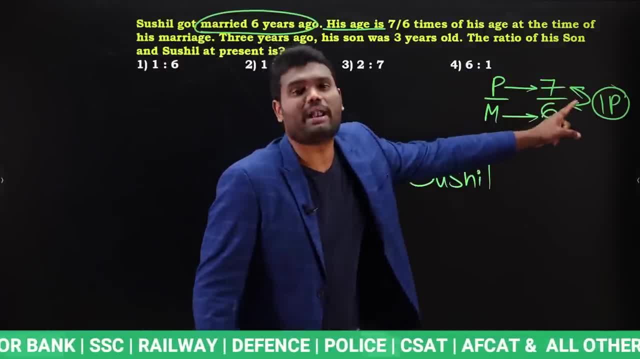 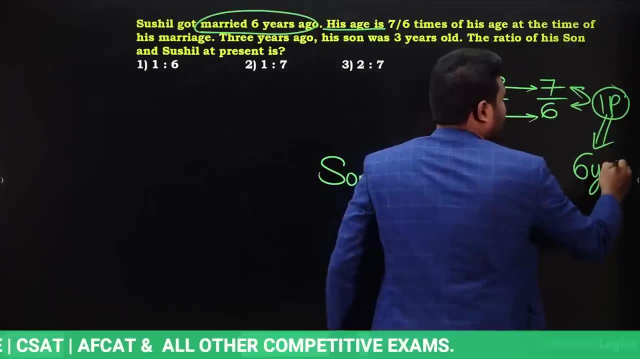 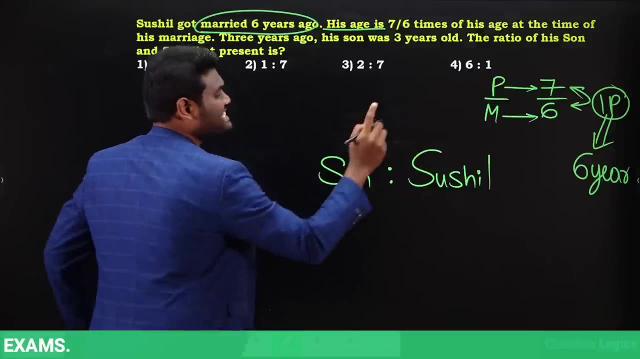 age difference in terms of parts is one part. Age difference in terms of years is 6 years. So one part is equal to 6 years. If one part is 6 years then I can say percentage of Sushil is going to be 7 parts. 7 parts means 7 into 6, that is going to be 42 years. So Sushil percentage is: 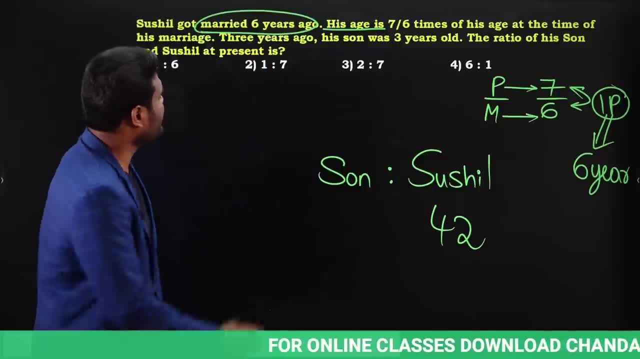 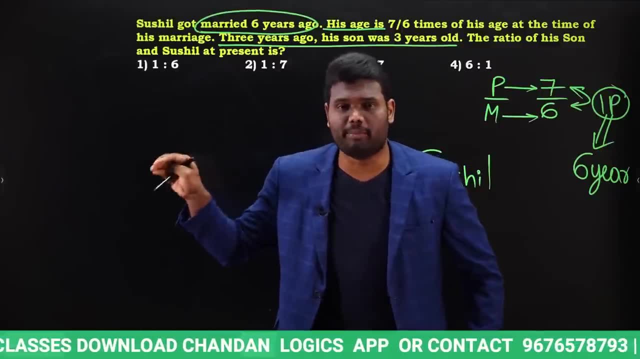 42 years. I need to know son percentage. In the question it is clearly said 3 years ago his son was 3 years old. 3 years ago his son was 3 years old means 3 years back, 3 years. Then what is the? 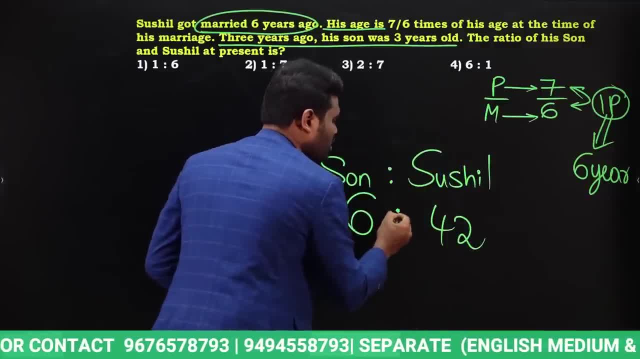 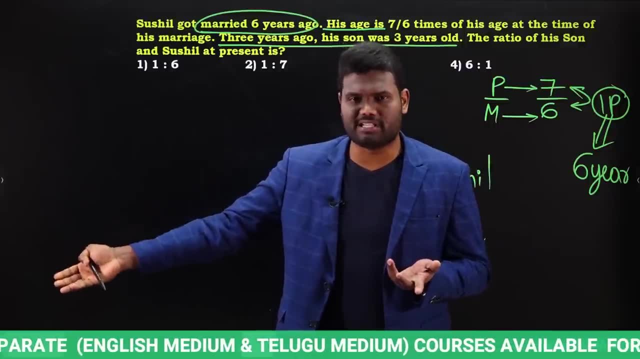 percentage: 3 plus 3, it is going to be 6 years, Yes or no? Let us say: 3 years back my age is 24 years. If 3 years back, my age 24 means now it is going to be 24 plus 3, 27.. Similarly, here, also 3 years. 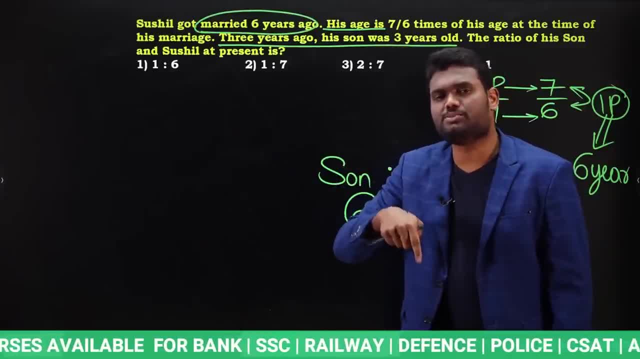 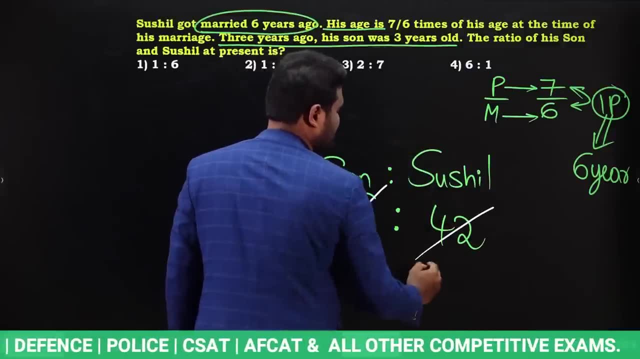 back. son's age is 3 years. Now will be. what is the age means? 3 plus 3, 6 years. Now calculate the ratio. If you calculate the ratio, what happened? 6 cancels here. 1 time. 6 cancels here. 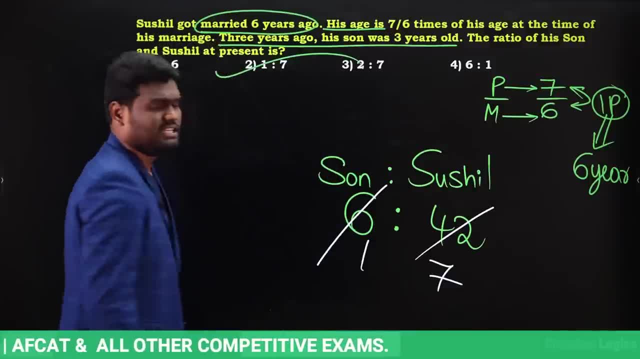 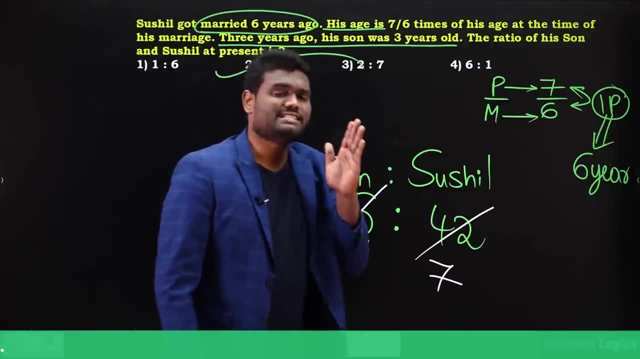 7 times. So ratio is going to be 1 ratio 7. Just a fraction of second. Complete information is given in the question itself. So it is very clearly mentioned that what is his age present and what is the age when he was got married? 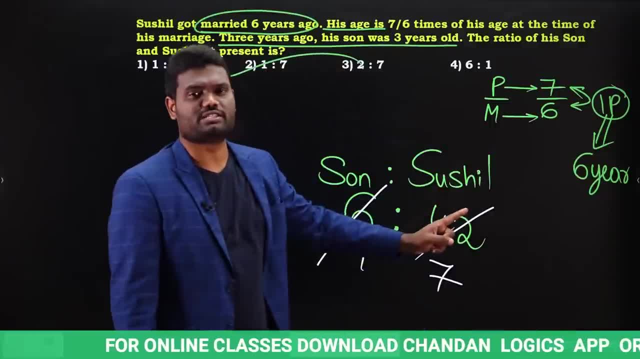 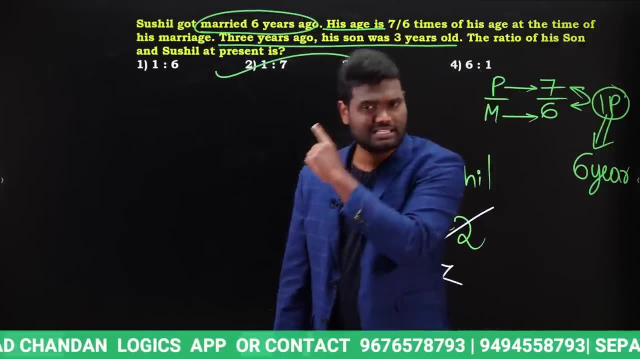 Ratio was mentioned very clearly. Ratio was 7, ratio 6, and it is very clearly said that he got married 6 years back, Which means difference in terms of parts is 1 part. Difference in terms of age is 6 years. 1 part is 6 years. If 1 part is 6 years, we are supposed to know. present is Sushil. 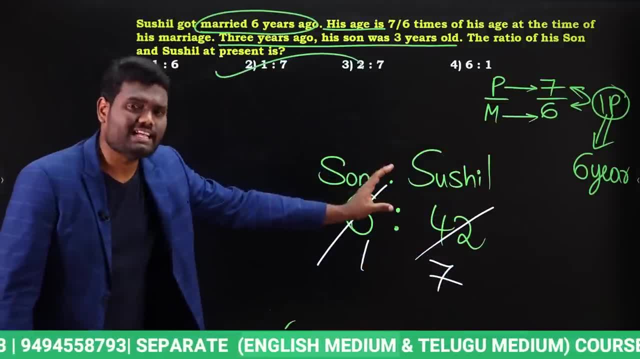 Present is 7 years. If 1 part is 6 years, we are supposed to know present is Sushil, Present is 7 parts. 7 into 6 is 42 years. So Sushil age present is 42 years. Sushil son age is nothing. 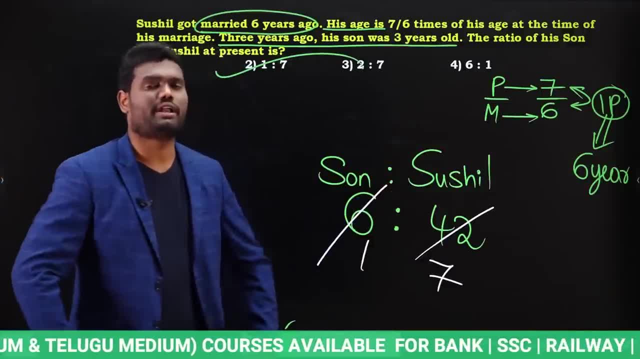 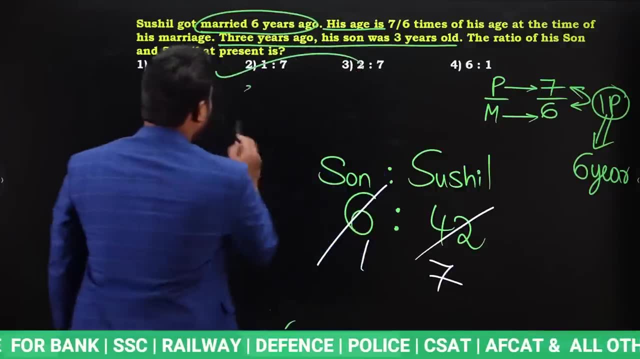 but 6 years, 6 ratio 42, which is same as 1 ratio 7.. Okay, Complete information given in the question. Now, without understanding the question, what many students will do? They will go on doing the rough work. No, you are not supposed to do that. Understanding the. 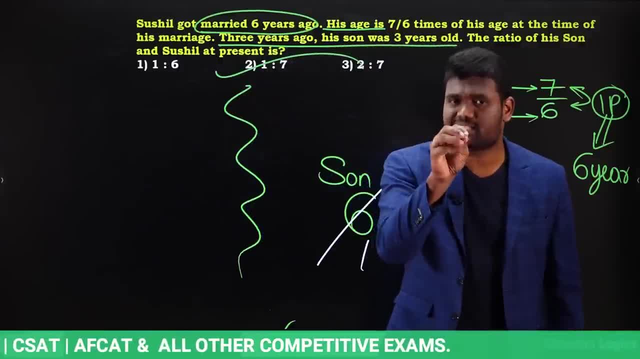 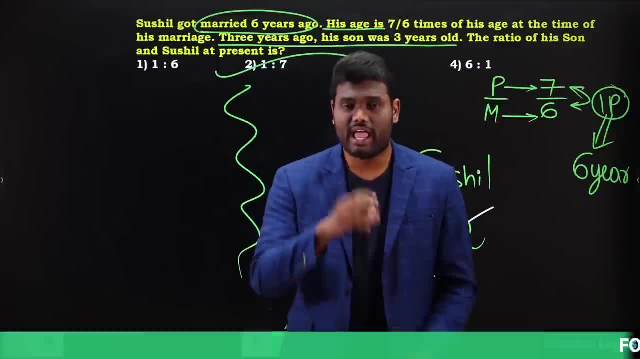 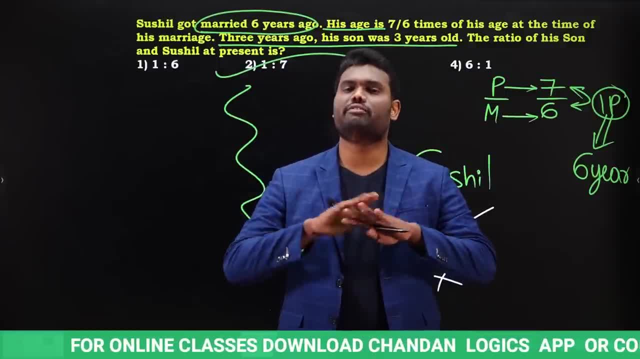 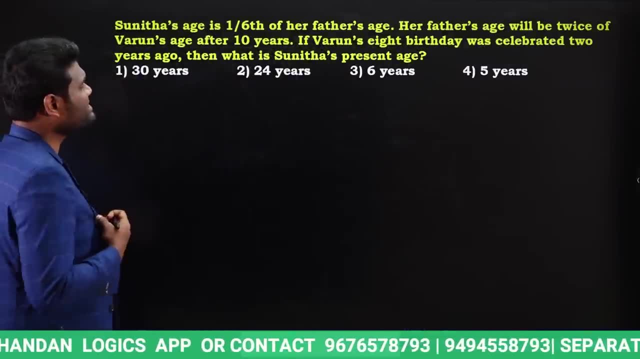 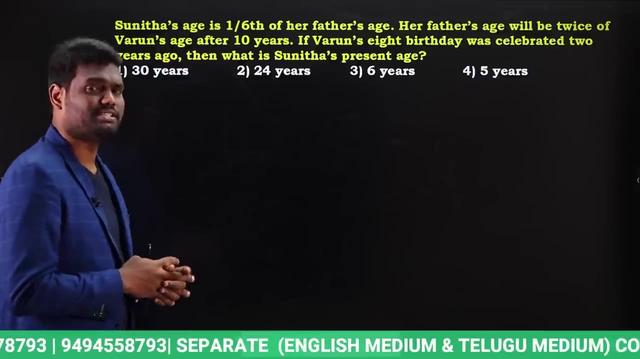 to understand the information that is given in the question, then obviously solving questions will be very, very simple. Okay, Let us look at one more question. Sunita's age is 1 by 6th of her father's age, Which means Sunita's age will be 1 by 6th of her father's present. 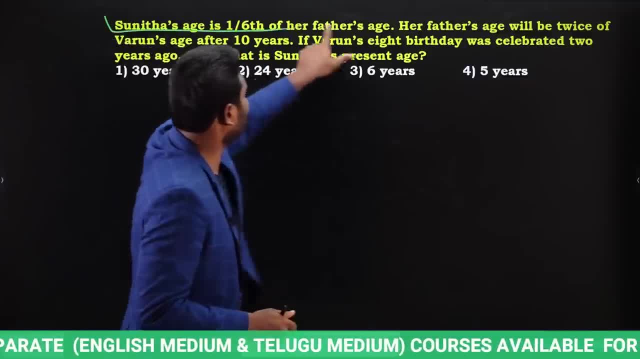 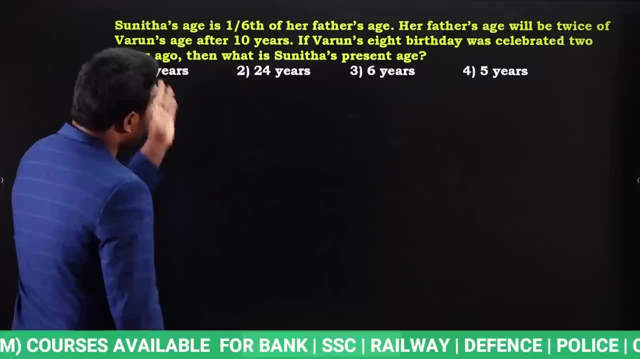 age. So nothing was mentioned means here there is no question. So you have to understand. information is about the present ages, okay, next, her father's age will be twice the twice of varun's age after 10 years. after 10 years, her father's age will be twice of varun's age, it seems. if varun's 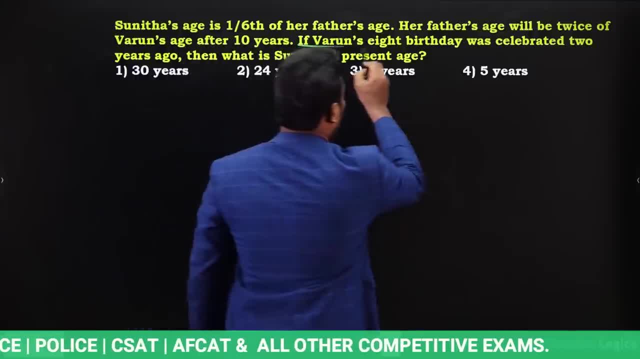 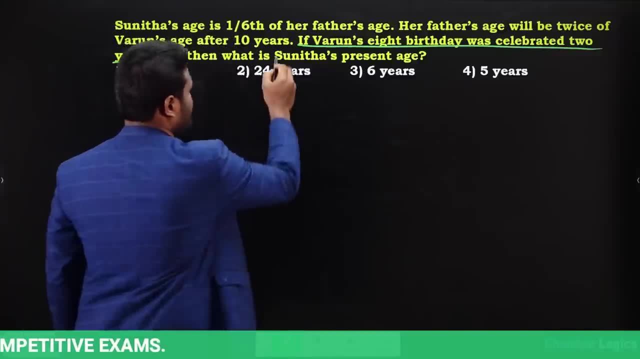 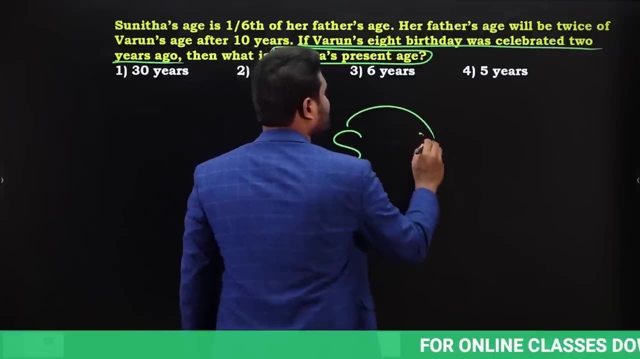 eighth birthday was celebrated two years ago. very important point. varun's eighth birthday was celebrated two years ago, then what is sunita's present age? so we had supposed to know sunita's present age. observe carefully in this question: if you need to find, sunita's age means first you. 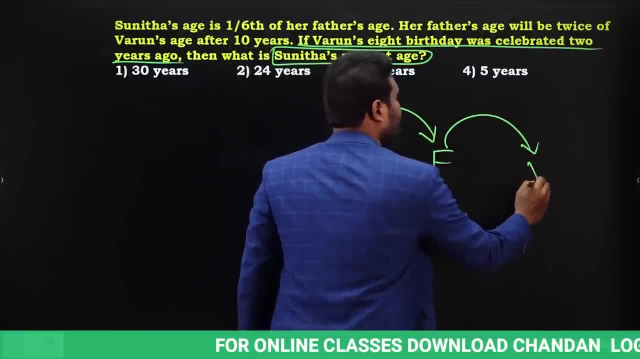 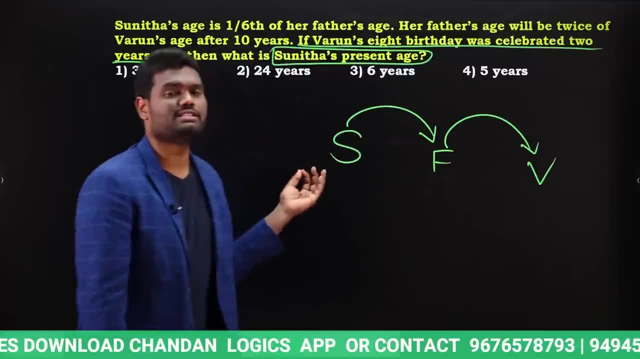 need to know father's age. if you need to know father's age means first you need to know varun's age. once if you know varun's age, based upon varun's age, you can say father's age once. if you know father's age, then automatically you can say sunita's age. yes, first of all try to know what is. 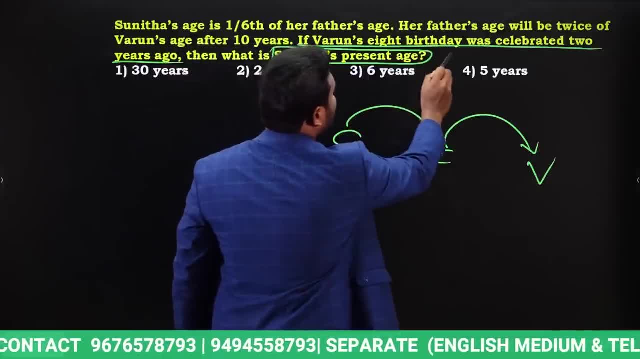 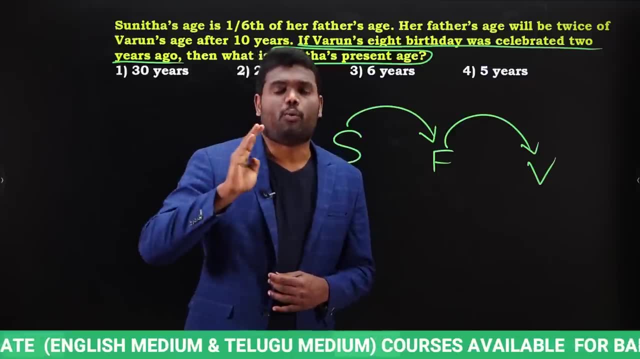 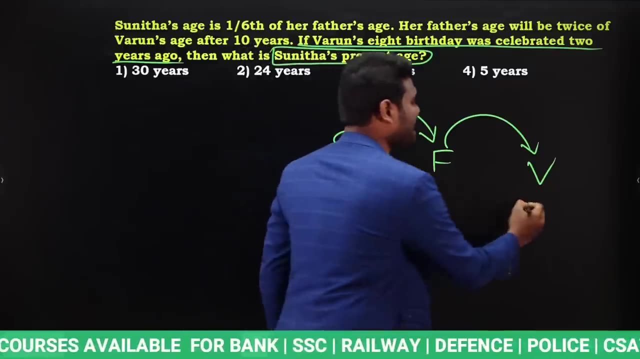 varun's age. it is very clearly said: varun's eighth birthday was celebrated two years ago, which means two years ago. varun celebrated eighth birthday means Varun's age was 8 years. when 2 years ago- 2 years ago- 8 years means present, it should be 8 plus 2. 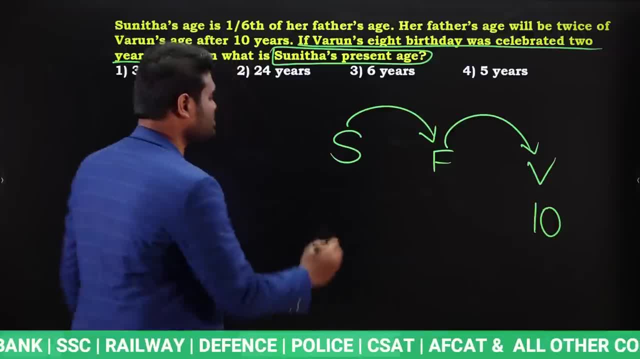 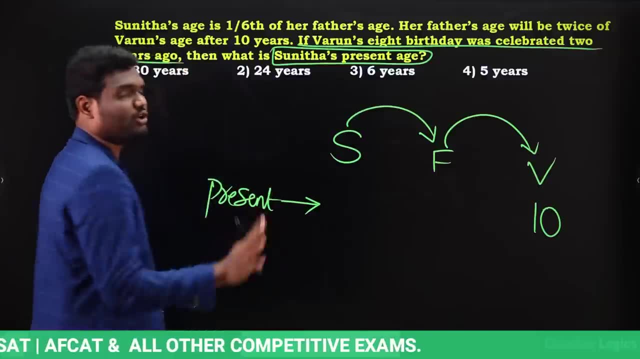 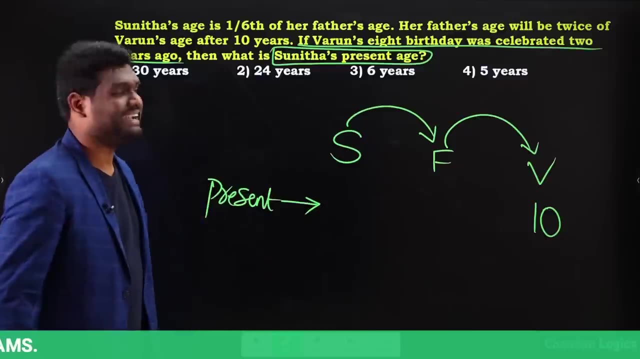 10 years. yes, which means Varun's present age is going to be 10 years. okay, Varun's present age. actually, this question can be done orally without using pen and paper, but, as you guys need to understand, that is reason I am using pen paper. okay, so Varun's present is going to be 10 years. 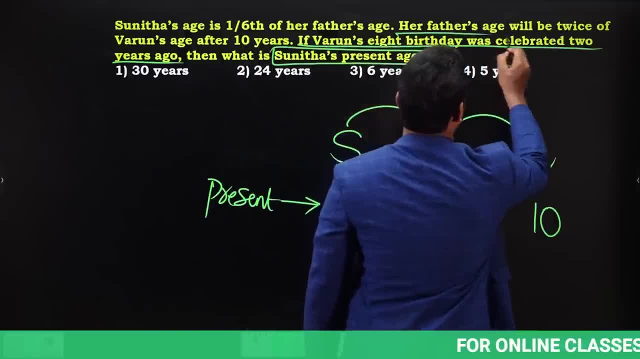 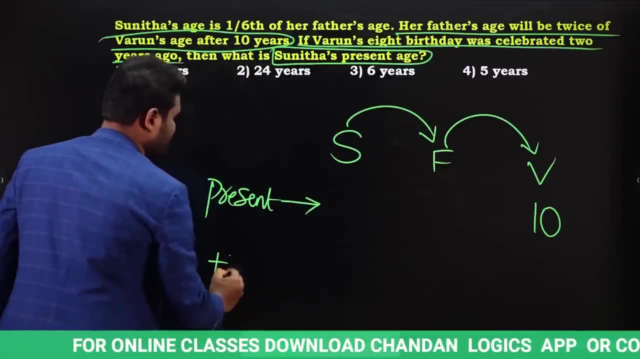 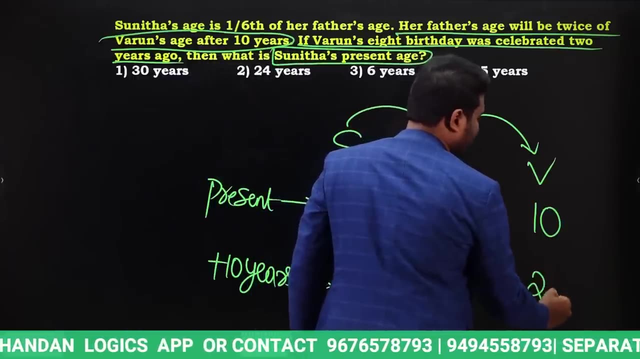 now what it is said in the question: her father's age will be twice of Varun's age after 10 years. now, present age is 10 years. means Varun's present age 10 years means after 10 years. after 10 years, Varun's age will be how much? 10 plus 10, 20? yes, if Varun's age is 20 means father's age should be. 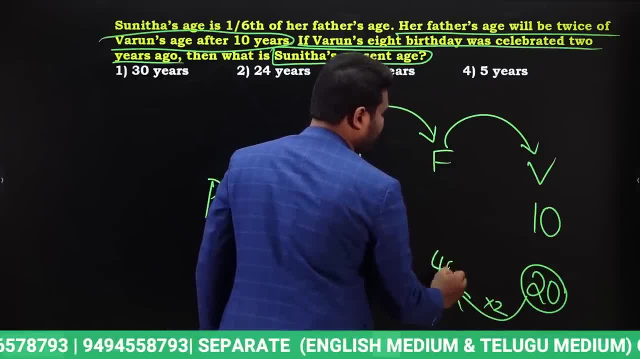 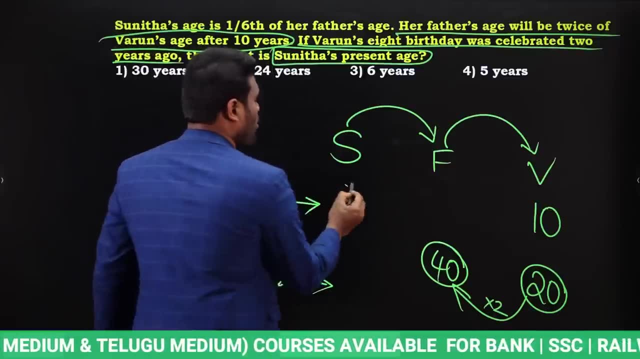 double. so father should double means 20 double that is going to be 40, which means father's age is going to be 40 years after 10 years. but we are supposed to know what is Sunita's present age if I need to know what is Sunita's. 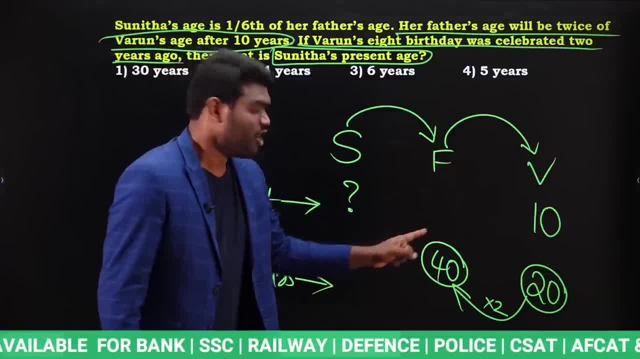 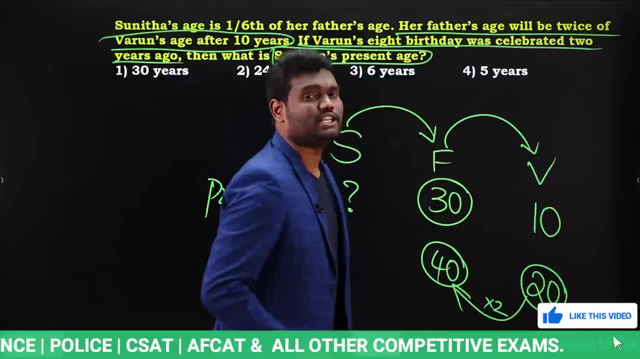 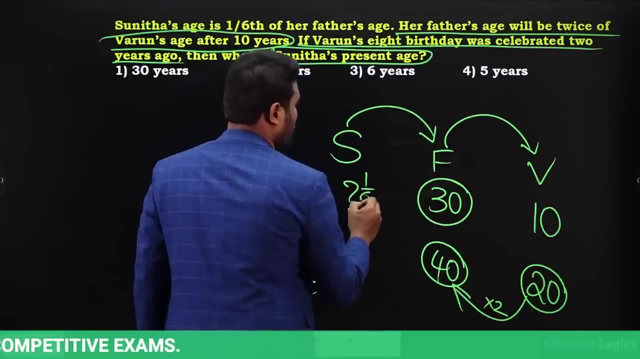 present age means, first of all I need to know what is father's present age. father's age after 10 years is 40. after 10 years, 40 means present age of father is going to be 30. present age of father 30 means it is very clearly said that Sunita's age is 1 by 6th of father. so 1 by 6th of father means 1 by 6. 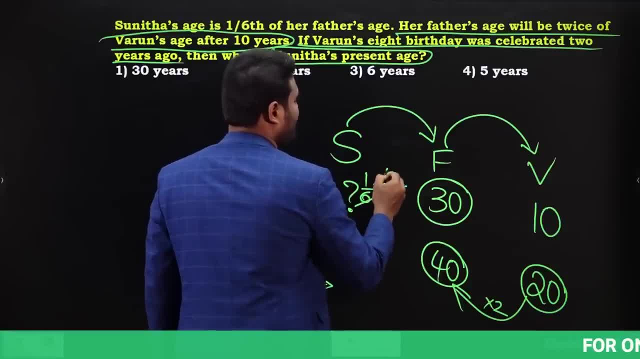 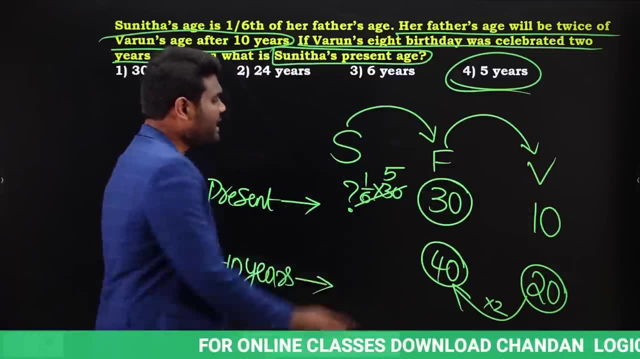 into: father's age is going to be 30. so 30 cancels in 6, how many times? 5 times, so we can say Sunita's present age is going to be 5 years. is that clear, very, very simple and truly speaking? all this information we need not write, but, as I was, 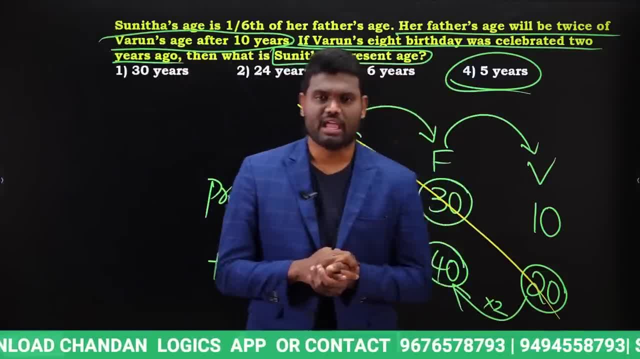 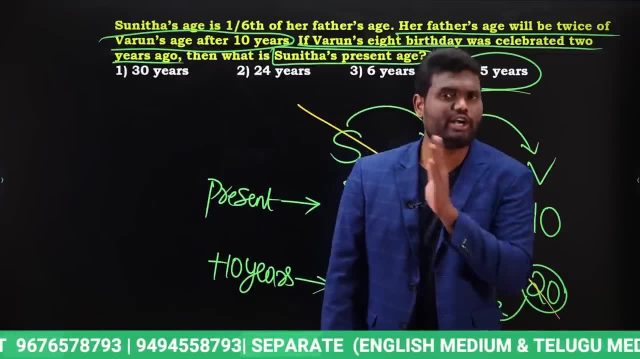 explaining you. each and every student should be clear. that is reason I have written very clearly, but this question can be done orally. if Varun celebrated his 8th birthday 2 years back means Varun's present day is going to be 10 years. if Varun's present day is 10 years means after 10. 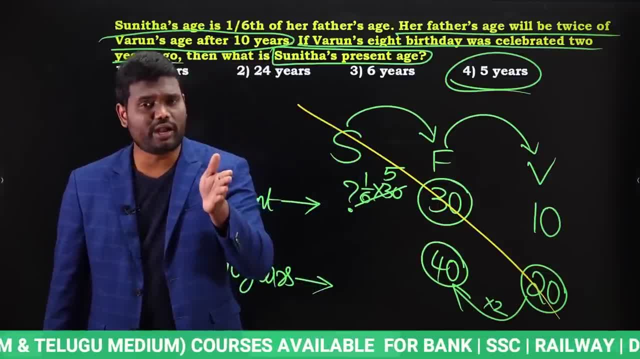 years, Varun's age will be 20 years and it's very clear that father's age is going to be twice of Varun's age after 10 years. so 20 years after 10 years means 20 years. after 10 years means 20 years. 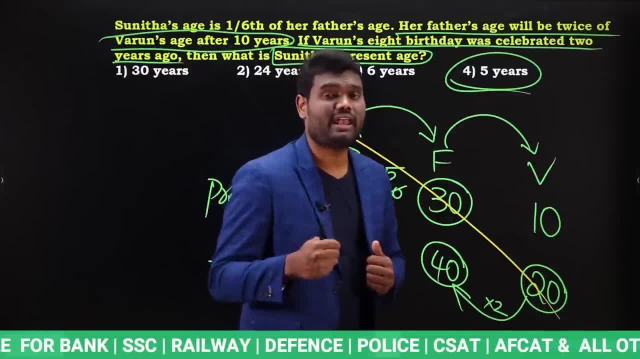 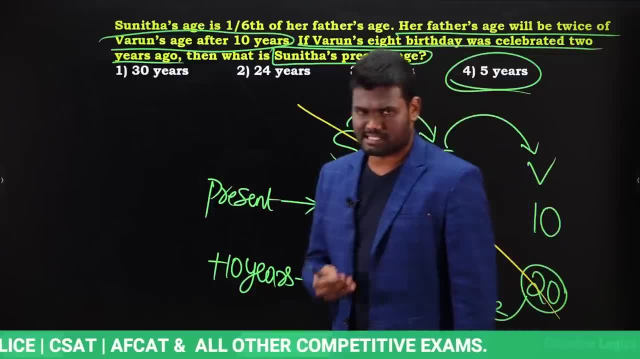 20 double will be 40, so father's age is going to be 40 years. when, after 10 years- after 10 years, 40 means present- it is going to be 30 years, father's present is 30 years. if father's present is 30 years, 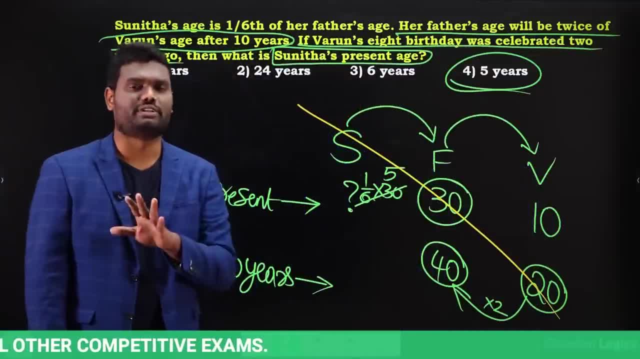 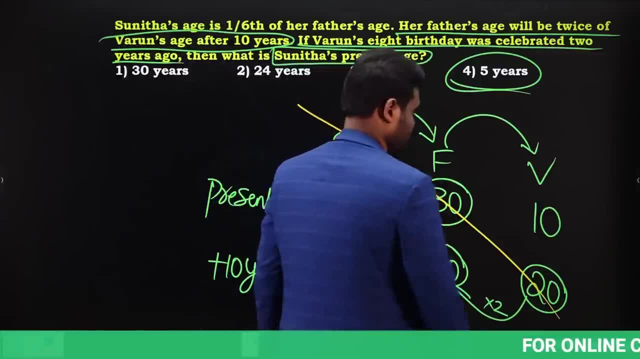 Sunita's age is 1 by 6th of father, so 1 by 6th of 30. 1 by 6th of 30 means 5, which means Sunita's present day is going to be 5 years. is that clear, very, very simple question? so let us look at one. 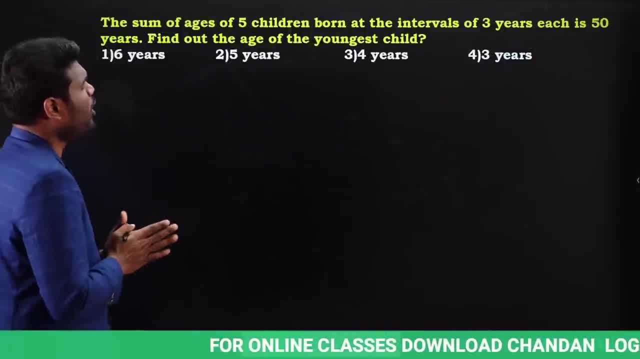 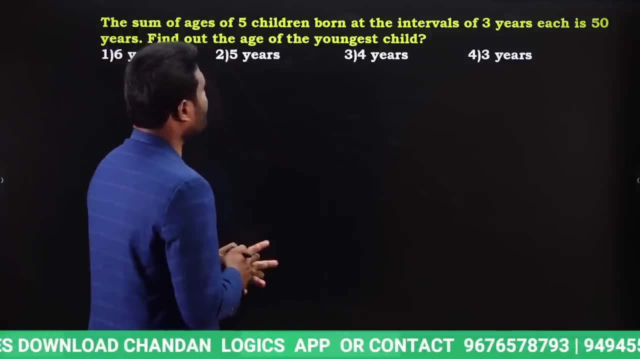 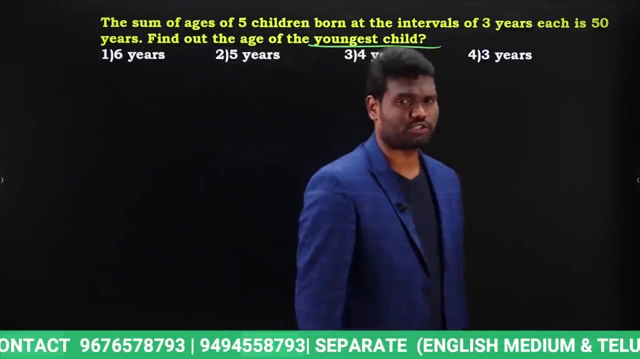 more question: the sum of ages of 5 children born at the regular intervals of 3 years is going to be 3 years. each is 50 years. find out the age of youngest child. so we are supposed to find the age of youngest child. actually. this question is also very simple question. you can just mark the. 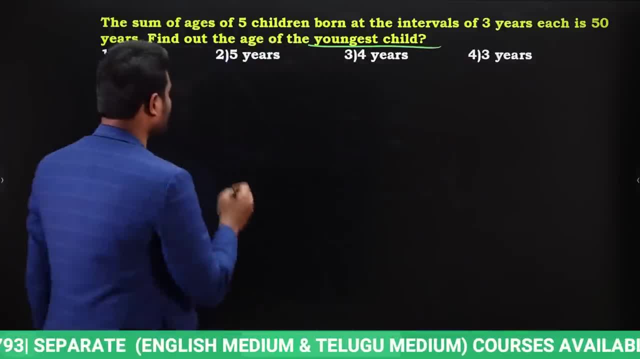 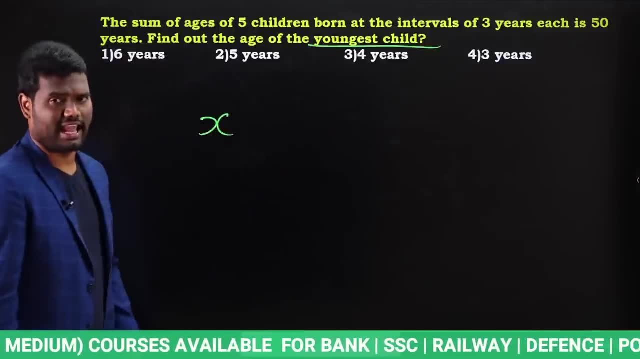 question in fraction of seconds, but what most of the students will do is like they will, as they does not know when the smallest child was born. they will take the smallest child as X after every three years. new child born, yes or no? so first child X means, next child X means next child X means. 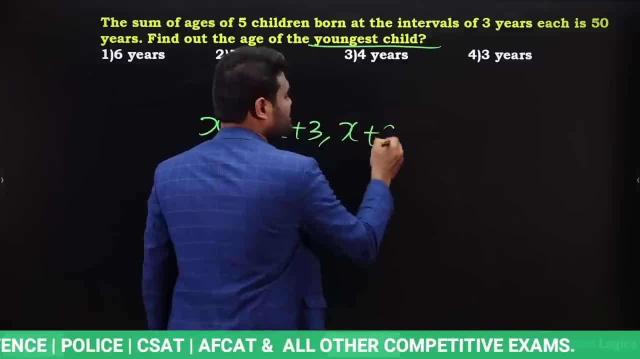 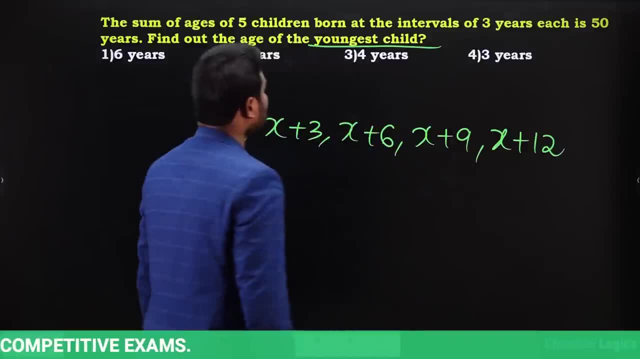 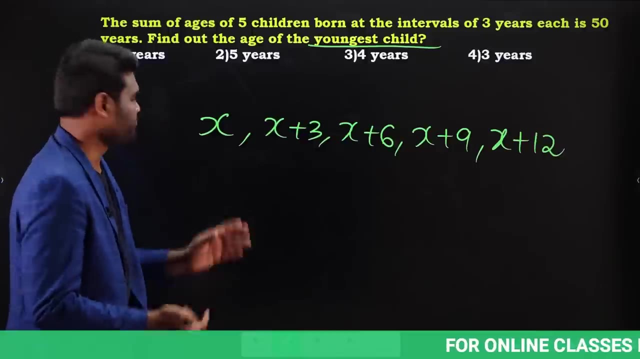 next will be X plus 3. next stage, it will be explained 6. next year it will be X plus 9. next, 陳, it will be X plus or 12. yes or no? total, how many children? five children, one, two, three, four, five. so total five children. everything is everything is new. child one: first year, the X years. 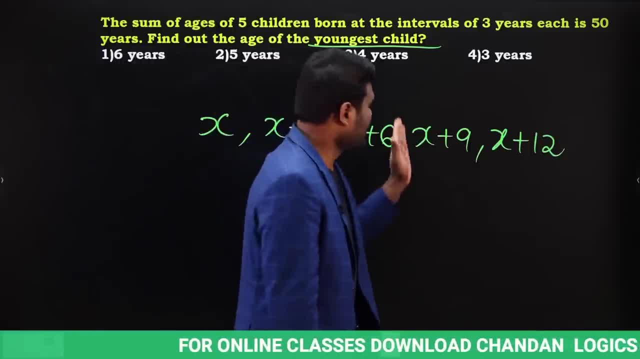 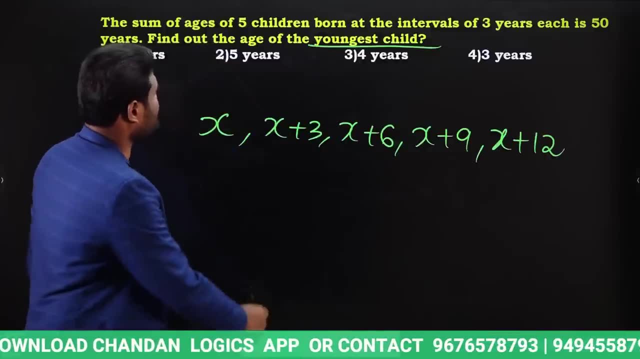 means: next year, X plus 3 years. next year X plus X years. next year, X plus on year's next year, X plus 12 years. yes or no? now what they're saying- some of their ages, some of their ages, they are of their ages- is going to be: how much Sum of their ages is nothing but 50 years. Now, what many. 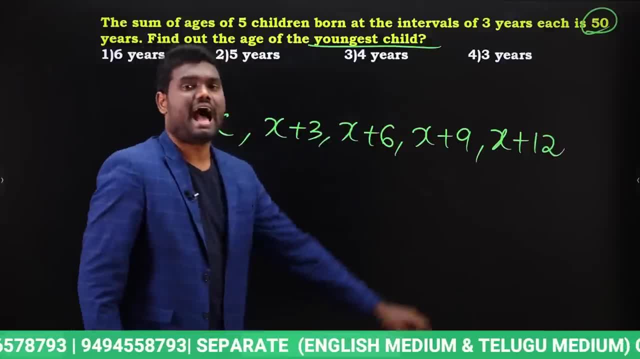 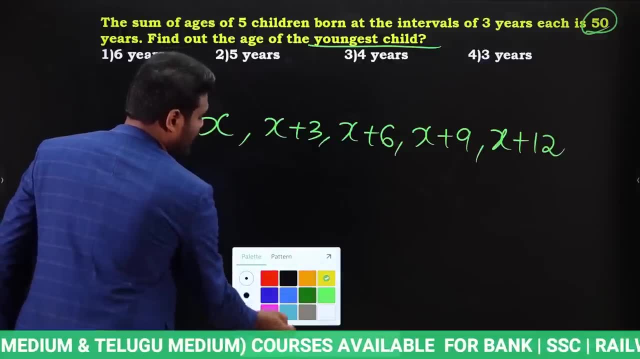 students will do. They will do sum and they will equal it to 50 and they will find the value of x and then they will say: what is the age of youngest child, Yes or no? Then they will say: what is the age of the youngest child? Yes, But truly speaking, if you are going to do this in examination, it is. 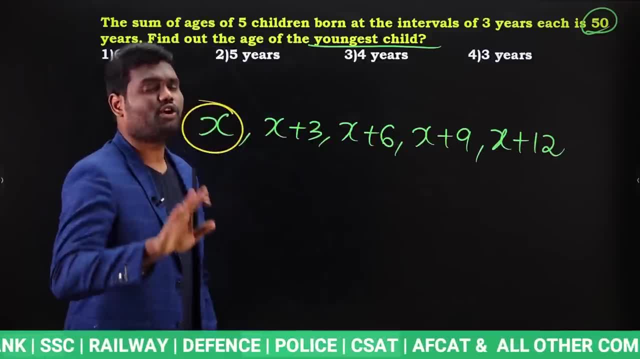 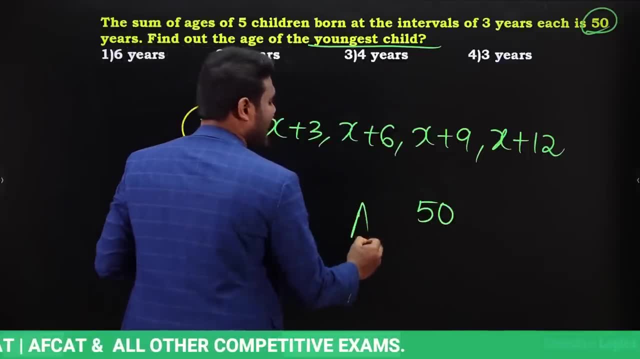 going to waste lot of time in examination. Yes or no? If you are really smart, it is very clear that sum is 50.. Yes or no? Sum is 50. If sum is 50, what is average? Average of 5 children is going. 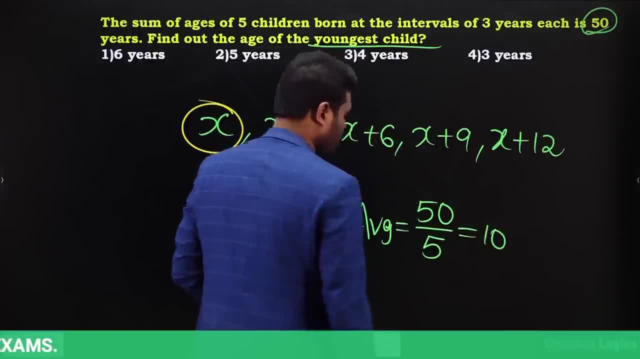 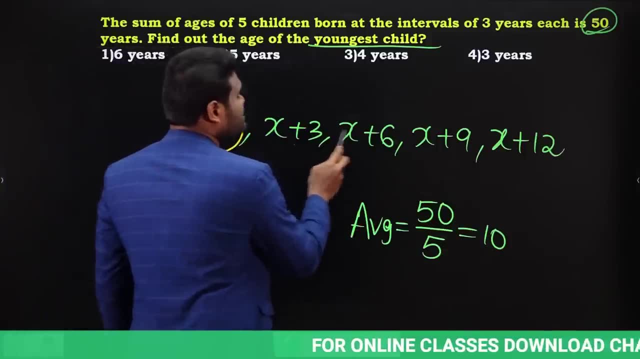 to be 50 by 5, that is going to be 10 years, Yes or no? Which means average of 5 children is nothing but 10 years. It is very clear that xi x plus 3, x plus 6, x plus 9, x plus 12- this is in arithmetic. 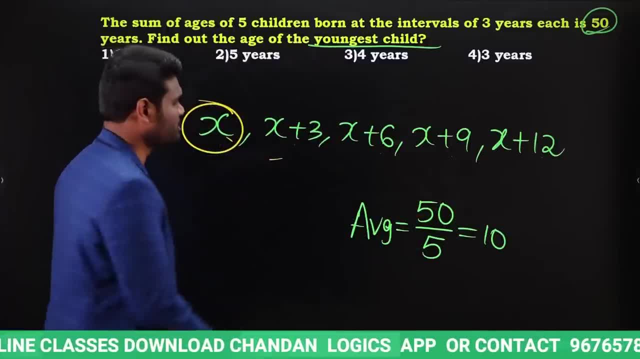 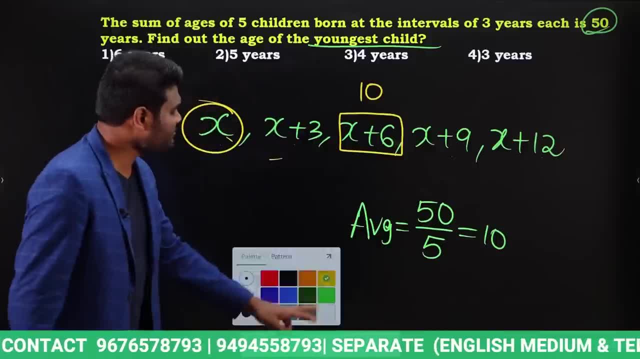 X plus 6 is nothing but 10.. If X plus 6 is 10, then what is the value of X? Value of X is nothing but 4 years, Yes or no? So you can directly say: answer is going to be 4 years. 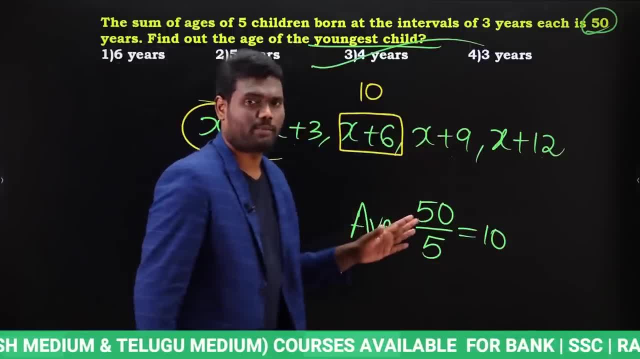 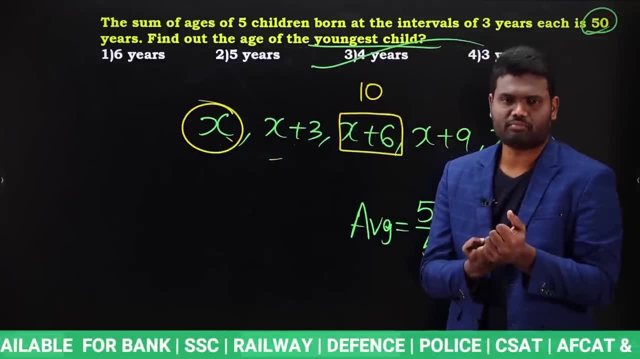 You need not calculate it, You need not elaborate it. Nothing is required. Commit to exams. No one will check your rough sheet- How much paperwork you have done. Will anyone check it? No one will check it After completion of your examination. you will throw it in the dustbin. 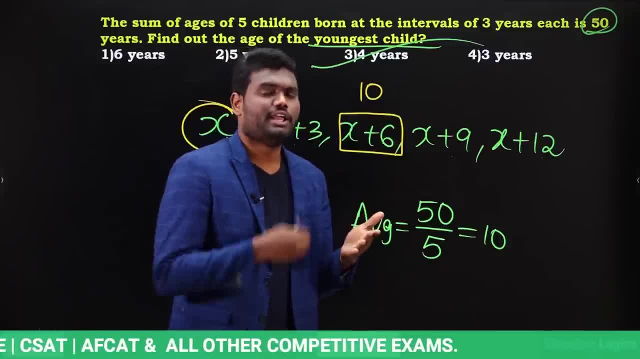 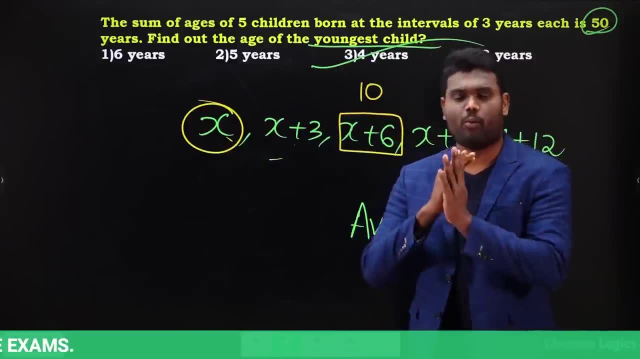 So always you have to avoid paperwork. If you have to avoid paperwork means definitely you have to be smart, Yes or no? If you are smart, only then you can avoid paperwork. So try to be smart, Try to be unique, So that you can avoid paperwork. 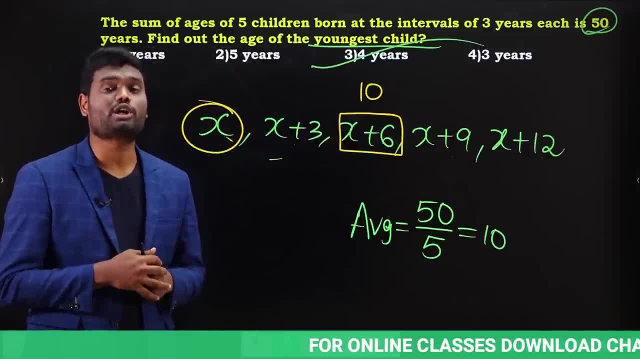 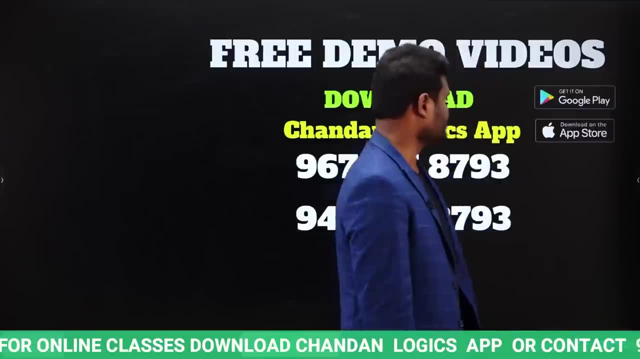 If you are going to avoid paperwork, then obviously you can save lot of time in examination. Is it clear? So answer for this question is going to be 4 years. Okay, So with this we are going to end the session, And if you are looking for more videos, you can download Sendan Noise app from Google Play Store. 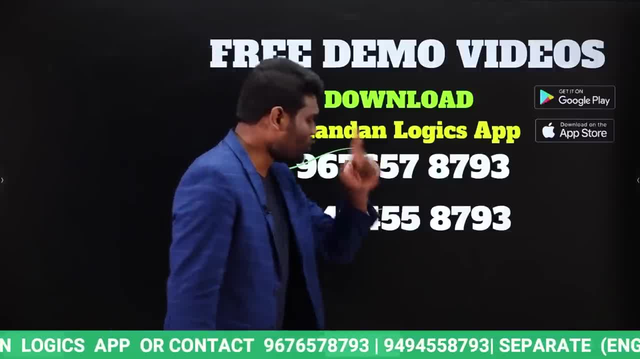 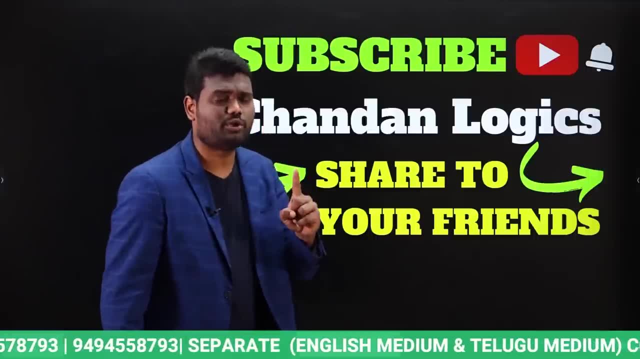 If you have any doubts, you can contact. And don't forget to like our video. if you like this session, And don't forget to subscribe to our channel. And if you like these videos, try to share these videos with as many friends as possible.